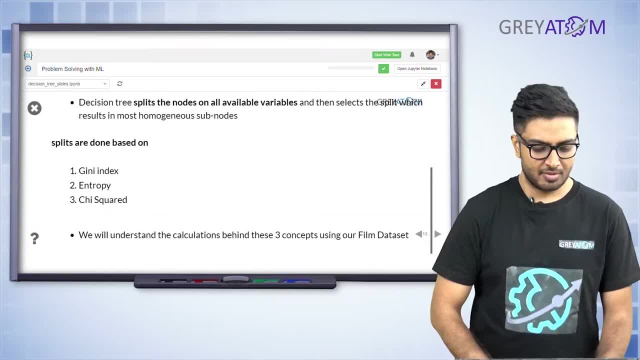 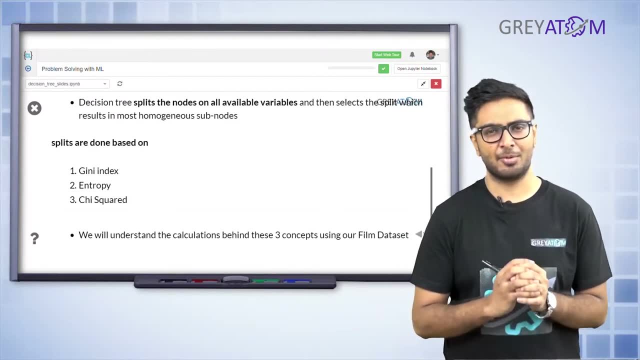 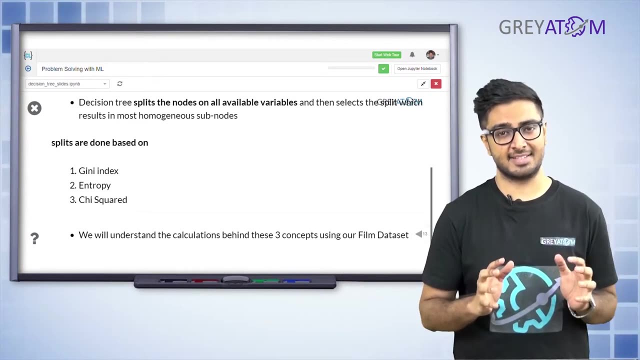 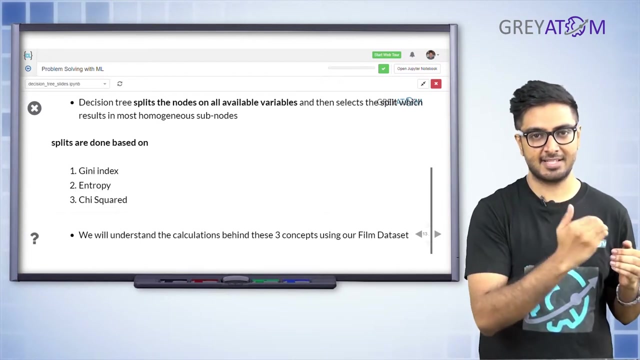 get a more better idea of that using Gini index. So there are three possible algorithms- Gini index, chi-square and entropy- and all of them are basically concerned about the same thing. The only thing that they vary among themselves is basically how they measure the impurity, But apart from that, the rest of the algorithms are exactly same. You have a node, you calculate impurity score, then, for all possible features, splits- you know, in this case gender split, employment split and age split- you're going to calculate the impurity of the produced nodes, right? 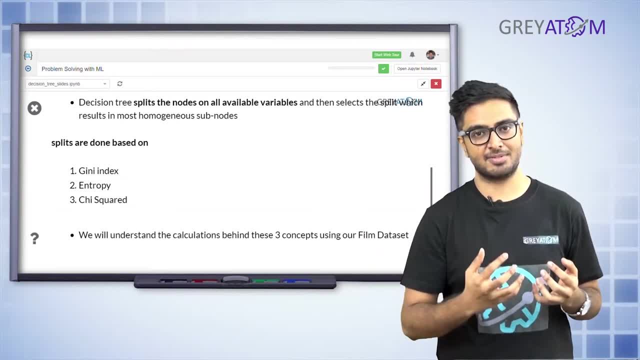 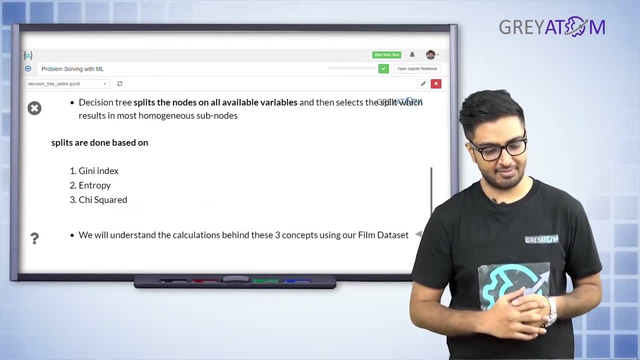 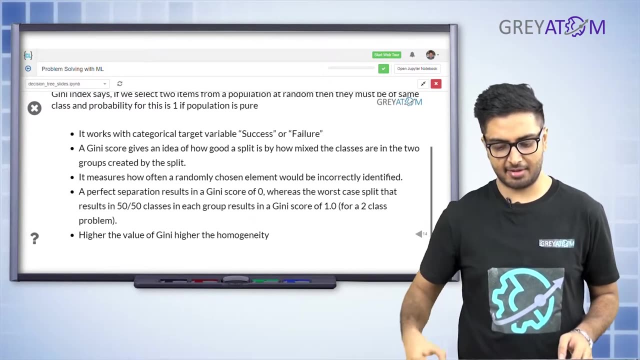 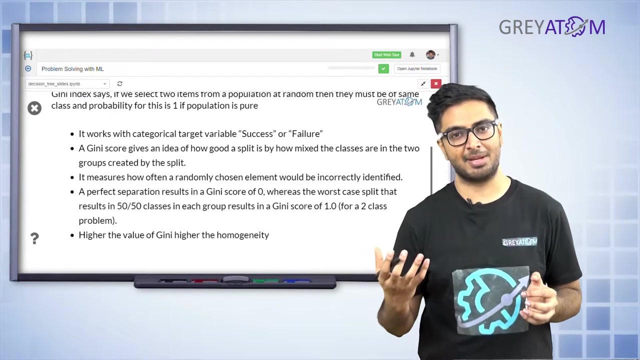 Whichever one gives you the least impurity score for the produced nodes, for the produced child nodes, you're going to go ahead with that feature. So let's try and understand that now using the dataset that we have. So the first idea is Gini index, right? So Gini index, how it is calculated, we are going to just go behind it. The main idea is if it's a measure of impurity. so basically, if you have a node which is extremely an impurity, you would have a score which is higher. If it's a node which is extremely pure, then you would have a score which is lower. And then the second idea: 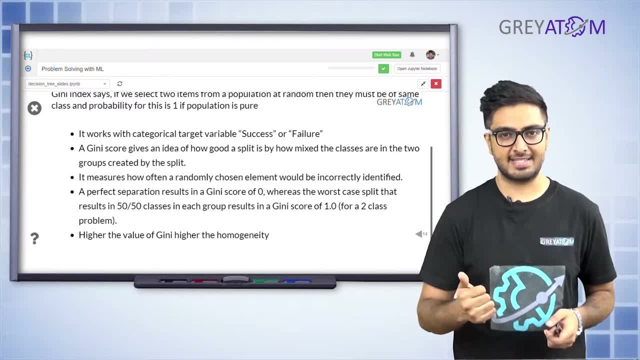 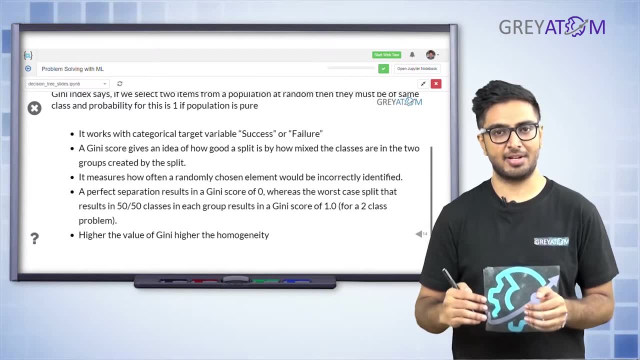 a genie index which is close to zero. but apart from that, that's exactly the whole idea of genie index and, for that matter, all the other algorithms is exactly same. you have an impurity score and that impurity score basically changes. uh, as you go, it goes decreasing as you go down the decision. 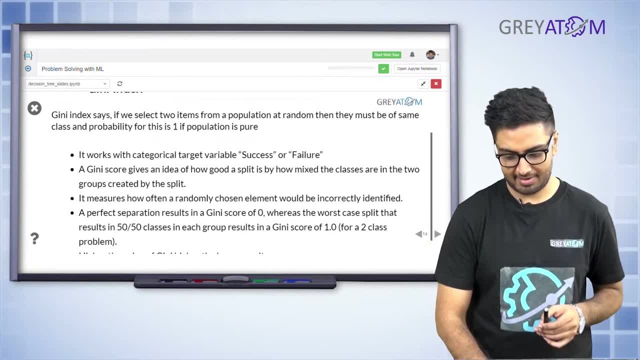 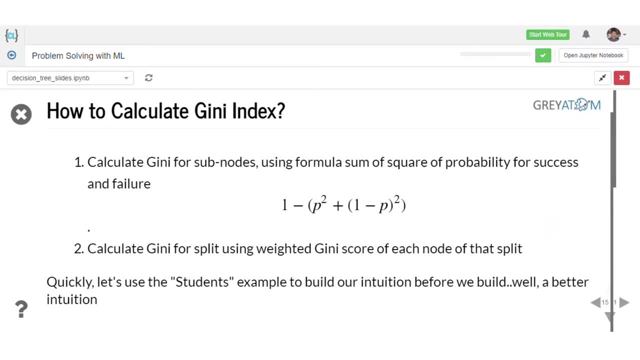 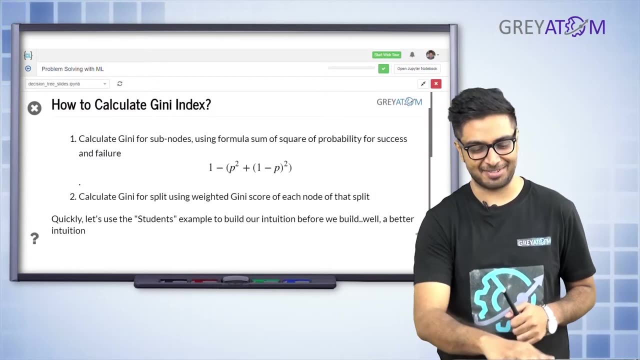 tree, right? so now let's have a look into genie index calculation, right? so what is the formula for genie index? say it says one minus p square plus one minus p square. right? so what? what are exactly all of this? and this sounds a lot more mathematical and all of this is complex, so let's. 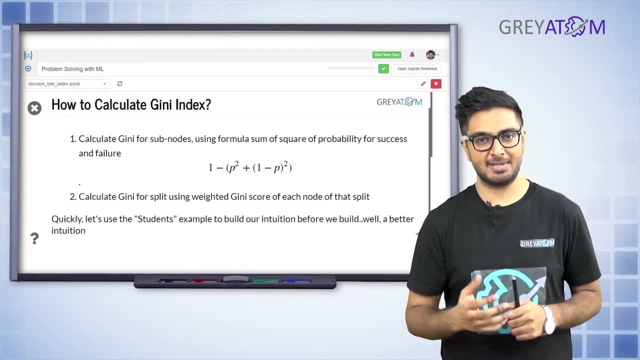 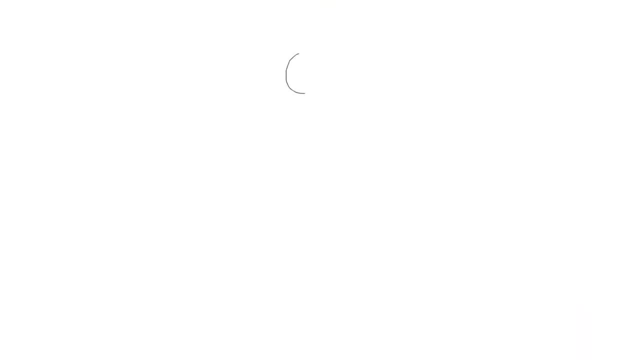 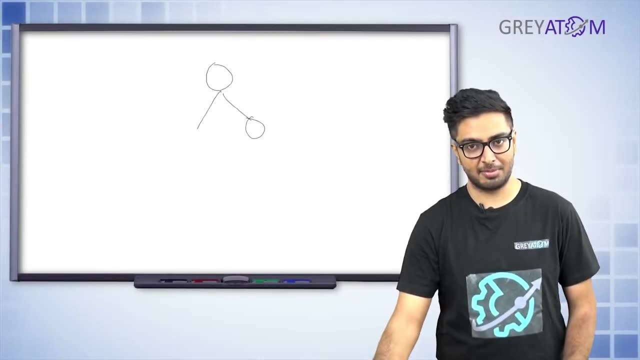 first understand what is p and what is one minus p. so p is basically the probability of success. so what is the probability of success? so, if i have? so this is the initial node and you have split that up such that here you have what is the probability of someone watching a movie, the probability. 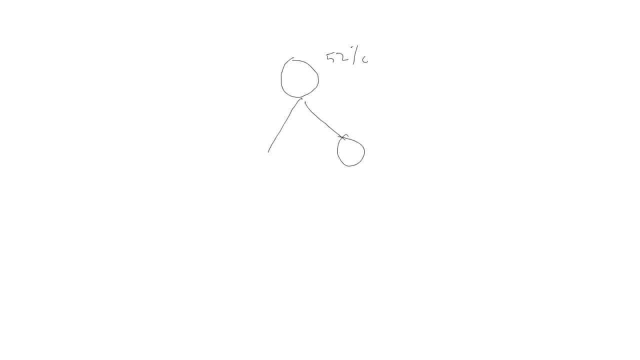 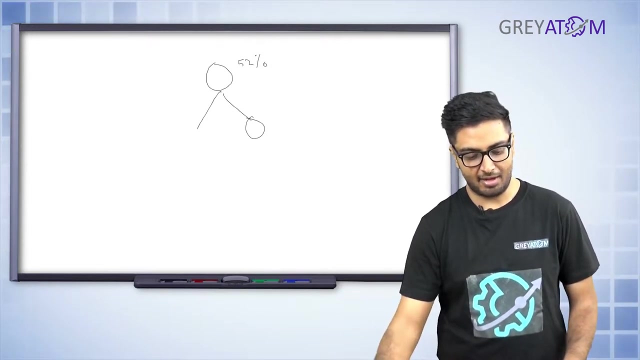 of someone watching a movie was 52 percent. right, we can we remember this? out of 50 people, 26 people have watched the movie. so probability of someone watching the movie is 52 percent. now, when we split it based on, say, age or something, there would be some probability of people watching the movie. 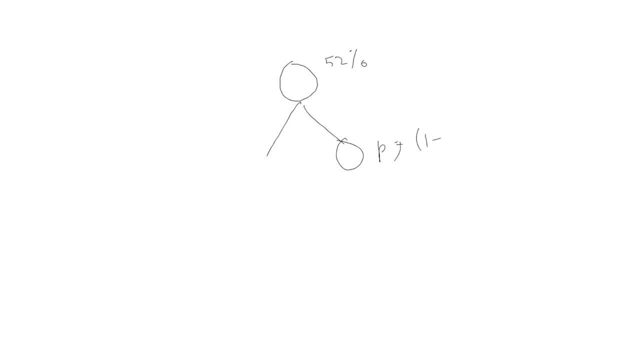 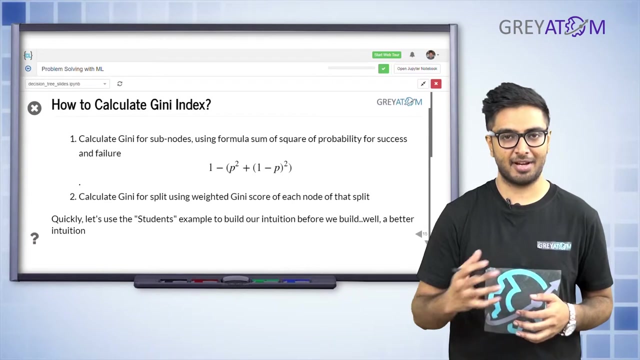 and there would be some probability of people not watching the movie. so, which is exactly 1 minus p, right? so that is the definition of p and 1 minus p. don't get so confounded by it right now. so let's, when we go ahead and we see more examples, the genie index calculation would be more apparent. 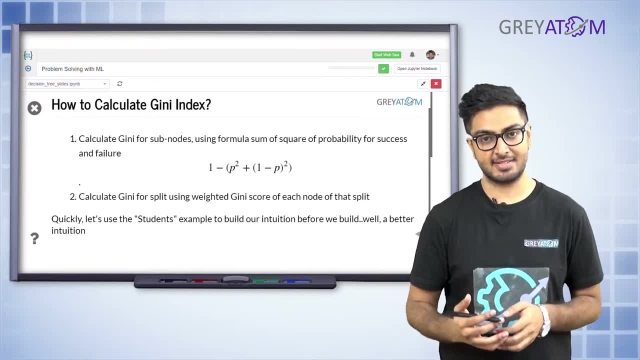 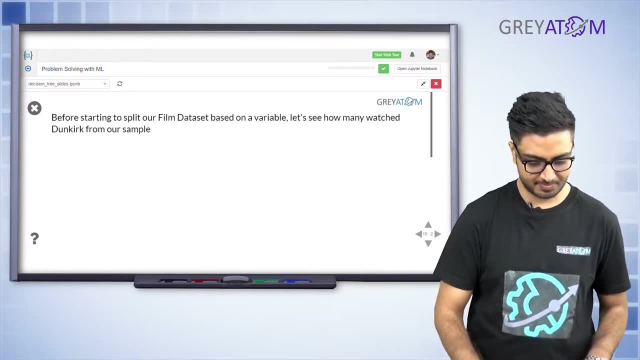 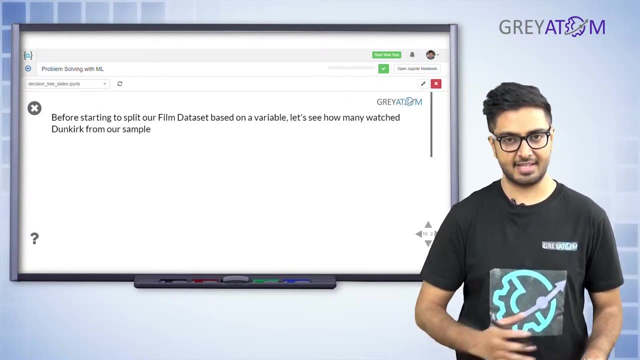 to you, and then that's when you should be able to appreciate why genie index is very high for an impure node and genie index value would be very low for a pure node, right. so now let's start building the intuition from the dunking data set that we have already looked at. 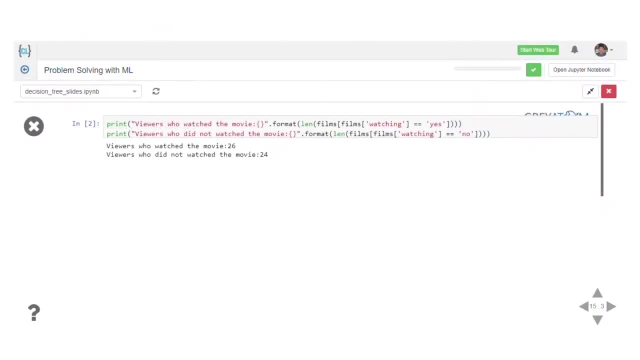 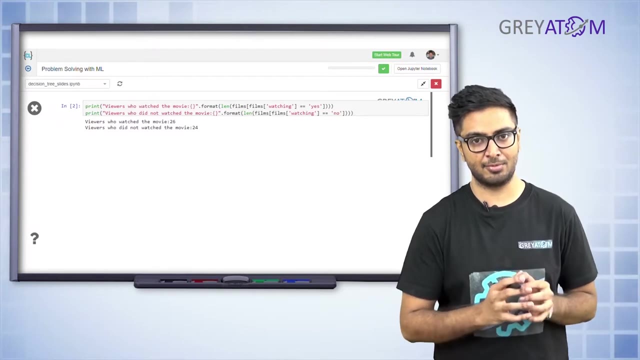 so first let's see how many people. so how many. what is? an number of people who have watched the movie is 26, so probability of someone watching a movie who in the root node is 52 percent and probability of someone not watching the movie is 24 into 248. 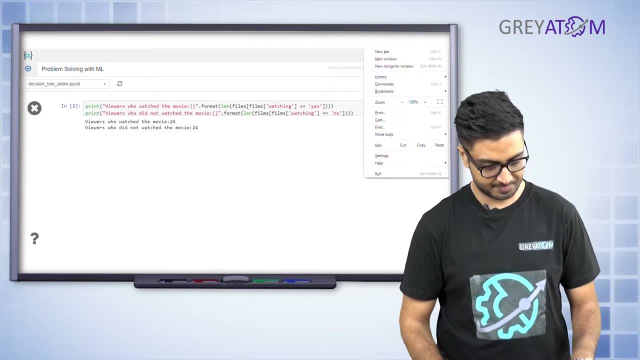 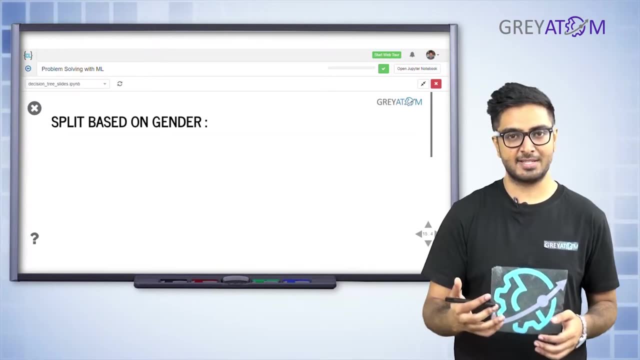 percent. right so now? so before we go ahead and go into looking at what are the different splits possible- split based on gender, split based on age and spit based on employment- and we calculate the genie index for each of those splits and the Finodor dela and sin insanely. 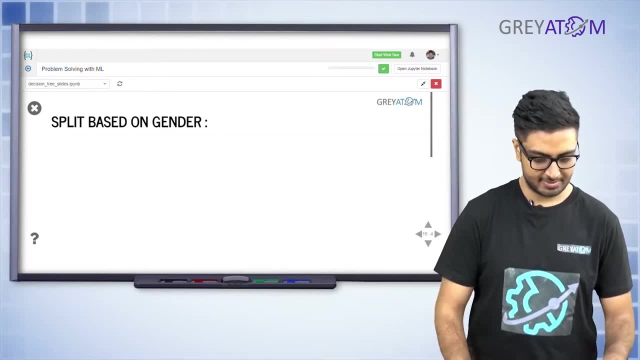 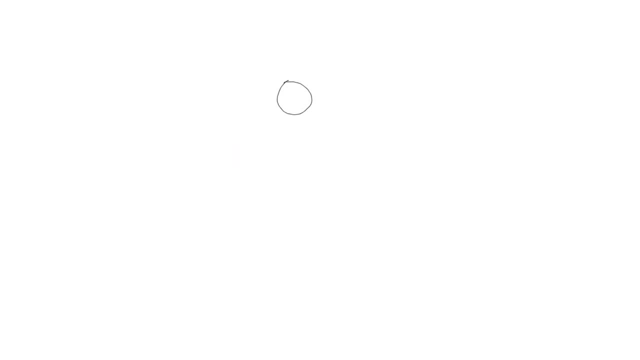 let's first try and calculate the genie index for the root node. so this is your root node looks like here. your probability of someone watching the movie is 0.52. probability of someone not watching the movie is 0.48. right, so genie index for you is 1 minus. 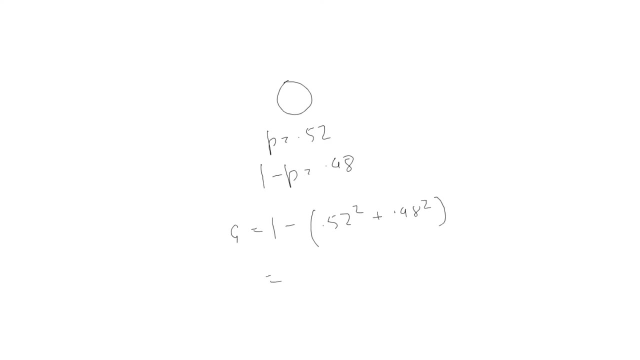 0.48 square right. so a month ago. all right, genie index for this original node. right the root. there's a root node, genie index right. so now let's try and take a moment and understand why genie index is a good measure of impurity now. 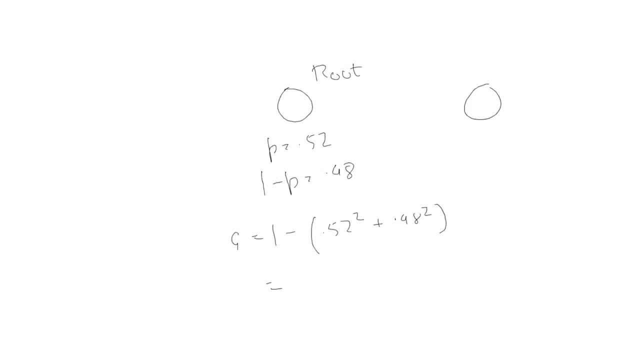 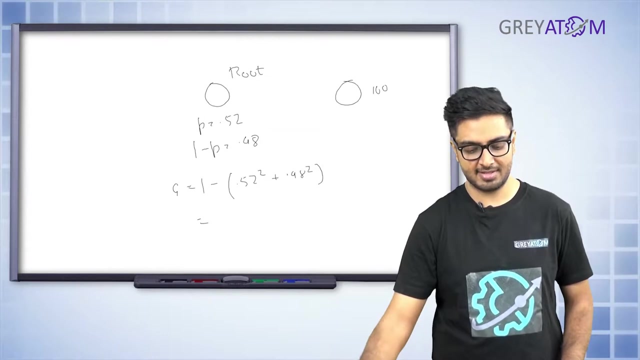 let's say you have a node which is completely where your everyone has watched the movie, right? so this root node- or even if it's not a root node, it's a child node or whichever node it is- has the probability where everyone has watched the movie, so probability of someone watching the movie. 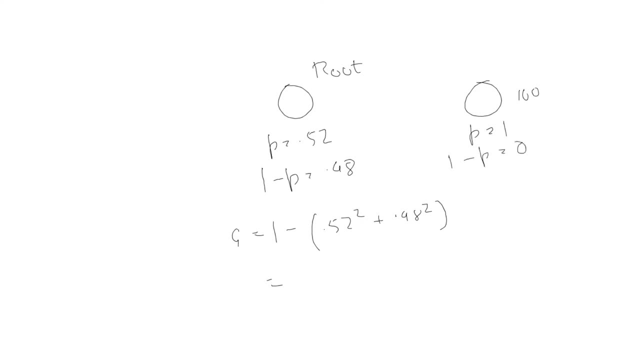 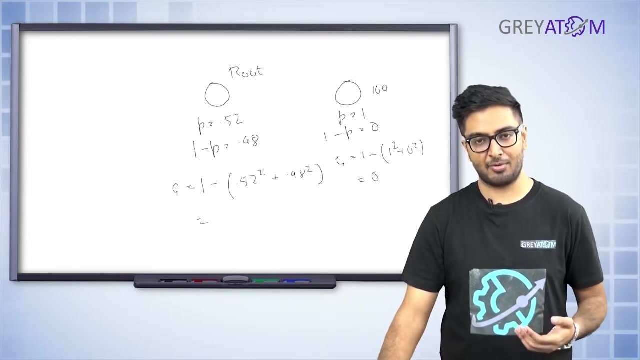 is 1, probability of someone not watching the movie is 0. and then your genie index is 1 minus 1 square plus 0 square, right. so genie index comes out to be 0. so you would be able to now appreciate: do the same thing, right? so if your probability of someone watching a movie is instead of 1, had it. 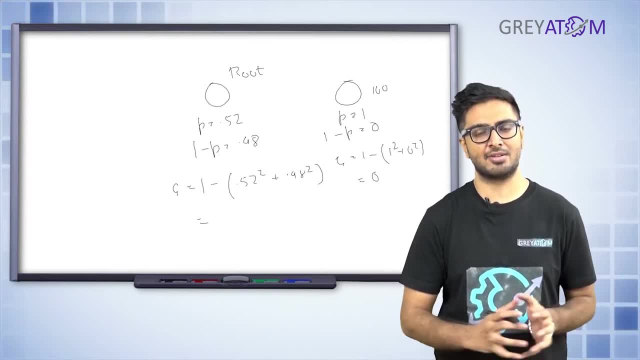 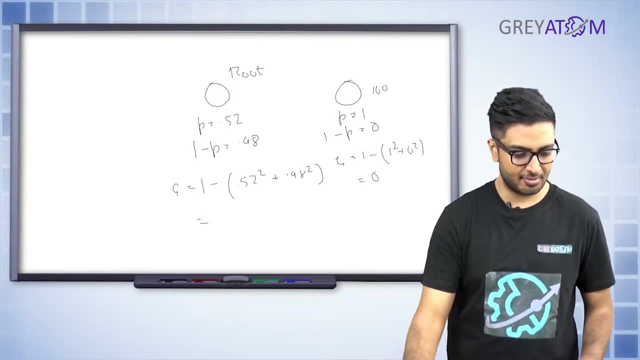 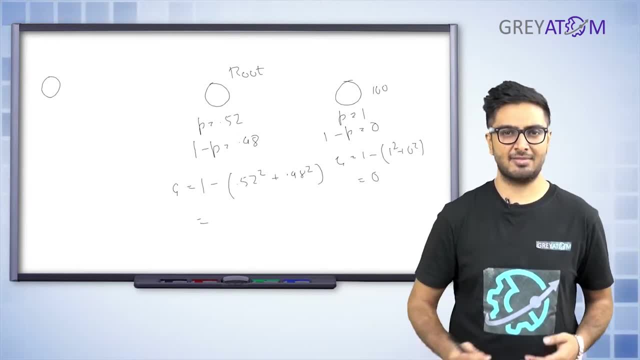 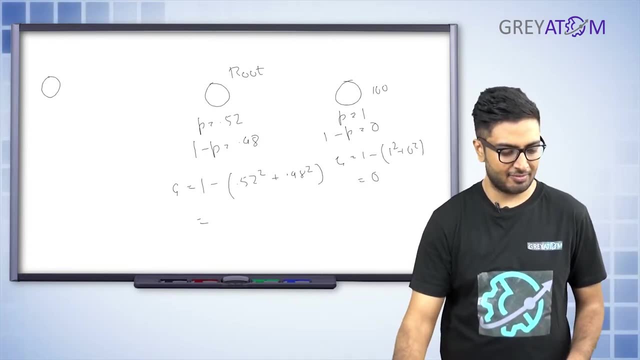 node which is extremely impure, right so, extremely impure, as in where it's exact 50 split, right so somewhat similar to the current situation we have. so we have a node where 50 percent of the people have watched the movie, so what is the probability of someone watching the movie? is 0.5, and then 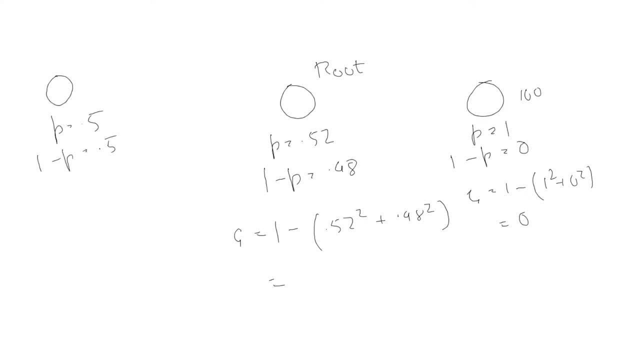 other 50 percent have not watched the movie, so that is an impure node, right? so now you calculate genie index. for them, g equals to 1 minus 0.5 square plus 1 minus 0.5 is 0.5 square, right. so this is 1 minus 0.25 plus 0.25, so this comes out to be 0.5. so for an extremely 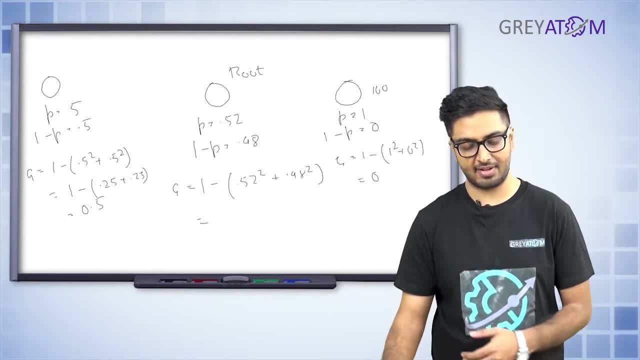 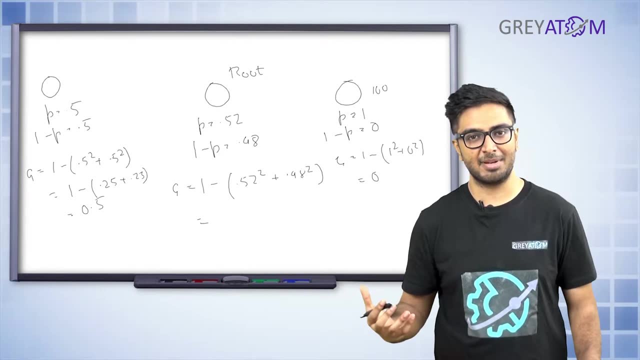 impure node, genie index value comes out to be 0.5, whereas for extremely pure node it comes out to be 0. so you can appreciate. so now you're able to appreciate this fact- that if it's extremely impure node, the genie index would be higher. if it's a very pure node or close to pure node, the 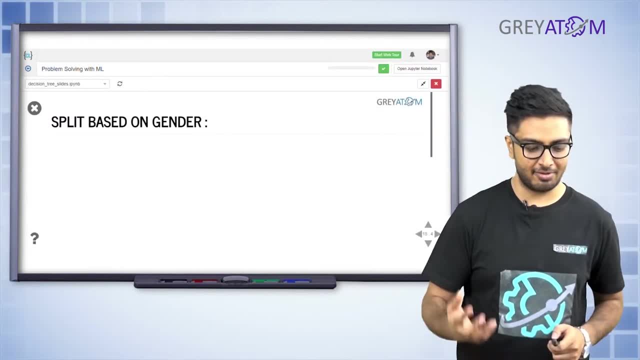 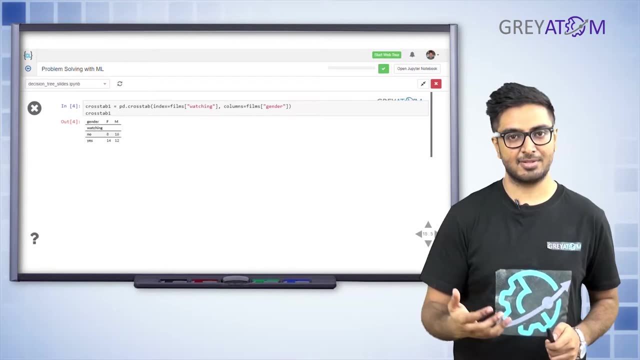 genie index value would be lower. so now you have that intuition. so now you have that intuition, so now let's do the exact mathematical calculation behind all of the possible splits and then we'll take a call based on those answers, which is the, which is the feature that we want to. 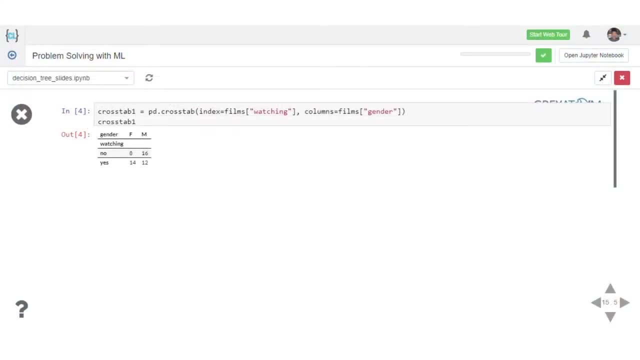 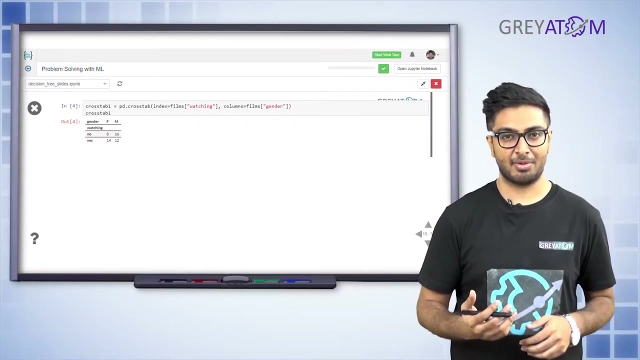 split on right. so the first up feature that we want to check is gender, right? so in gender, as i've explained you, there are 22 males and 28 females out of those 22. sorry, there are 28 males and 22 females out of 28 males. 12 people have watched the movie, so probability of someone. 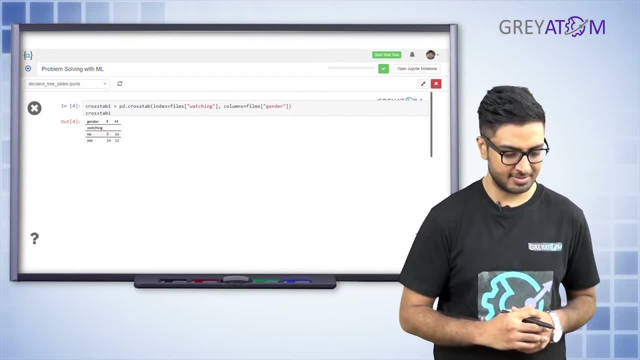 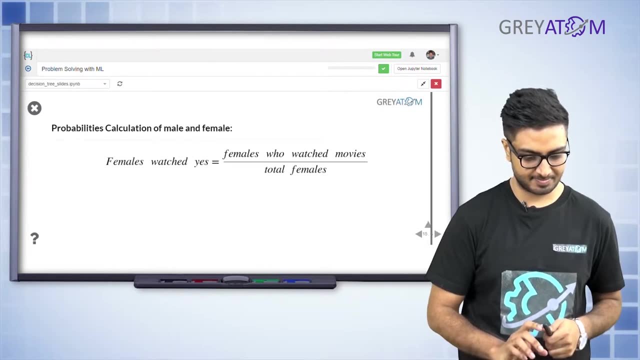 watching the movie is roughly 0.5. so that's the probability of someone watching the movie is roughly around 42 percent. and among females, 14 out of 22 people have watched the movie, so that's roughly around 63 percent. so now let's calculate the probability. so probability of a female who has 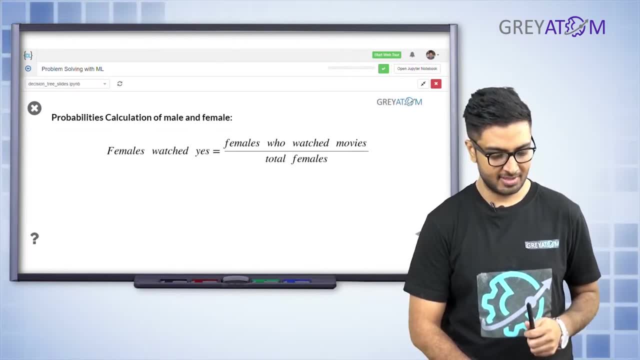 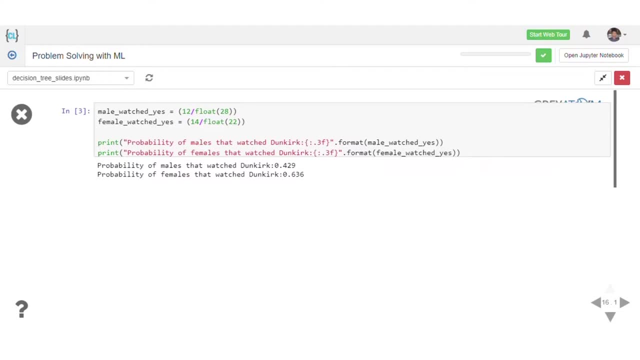 what is the probability that someone is a female and has watched the movie? that is yeah, so probability is someone who is a male and who has watched the movie. so that is 12 out of 28, which is 0.429. and what is the probability someone who's a female and watch the movie? that is 14 out of. 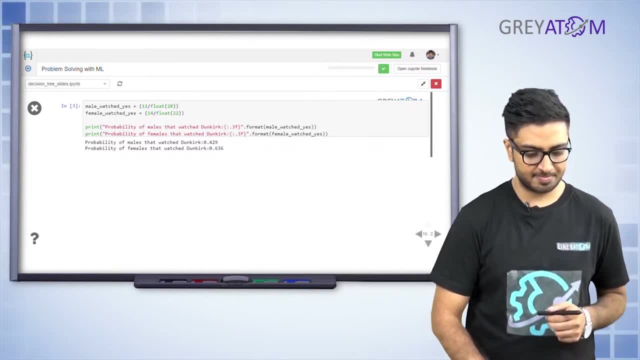 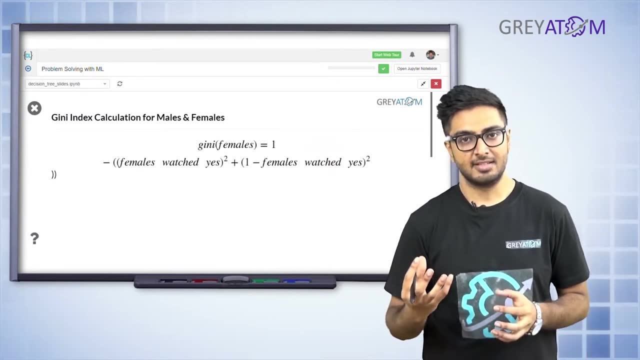 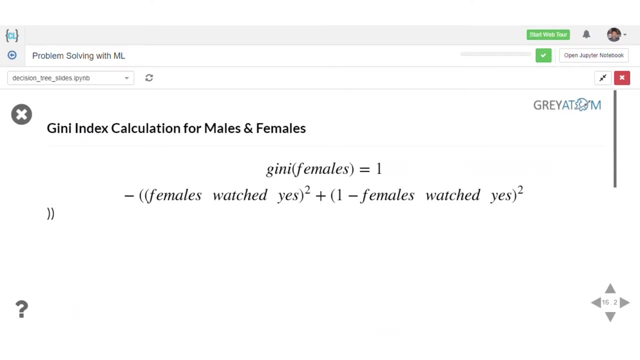 22, which is 63 percent right. so now, how do you calculate the genie index for each of the sub nodes? because genie index is calculated as a for each of the child nodes that are being produced. so genie index for females would be one minus probability of someone among females watching. 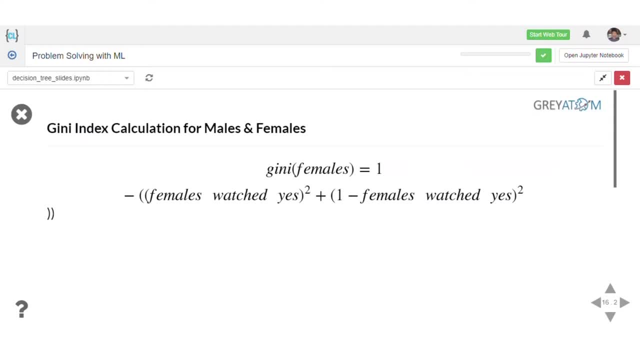 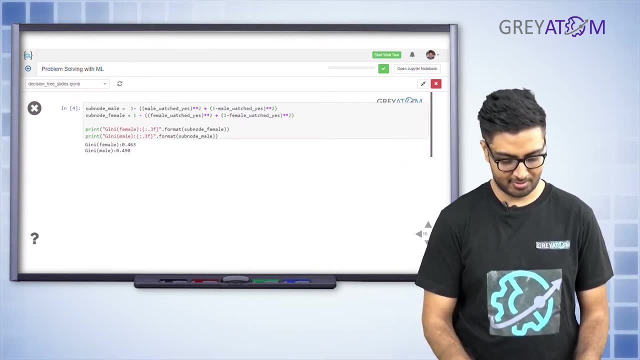 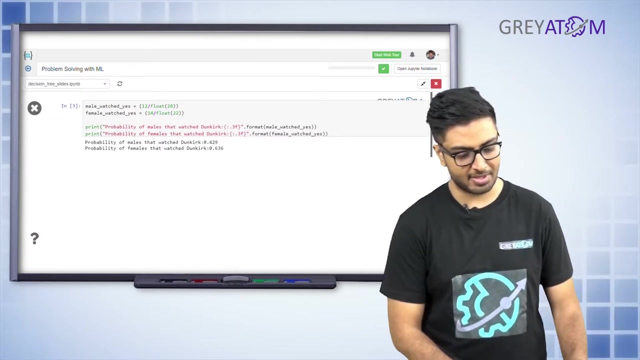 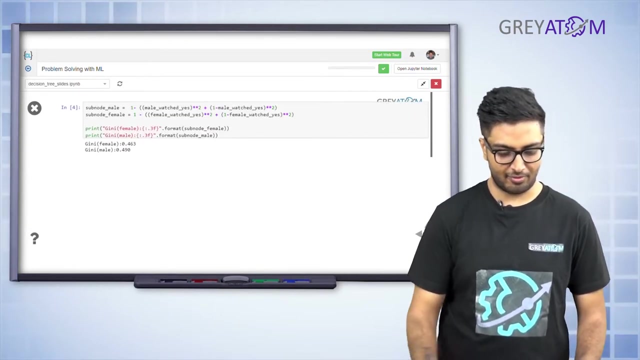 the movie. minus plus square plus one. minus that probability, square right. so what was the probability of someone watching the movie among females? it was 0.42, nine right, 0.43 around. that's what it is. yeah, so problem, sorry. probability among females having watched the movie. so p equals to 0.63. so your formula would be something like this: right, so 1. 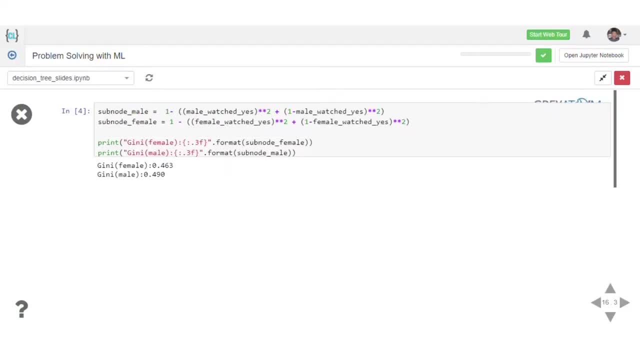 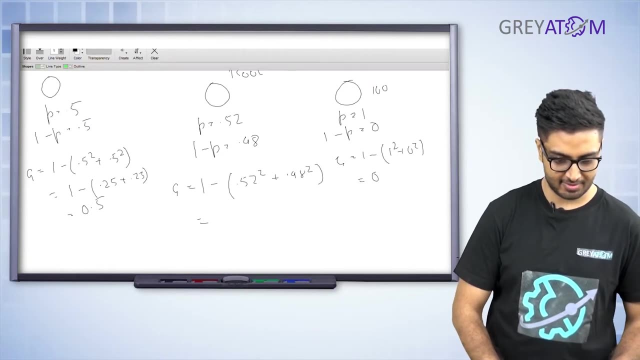 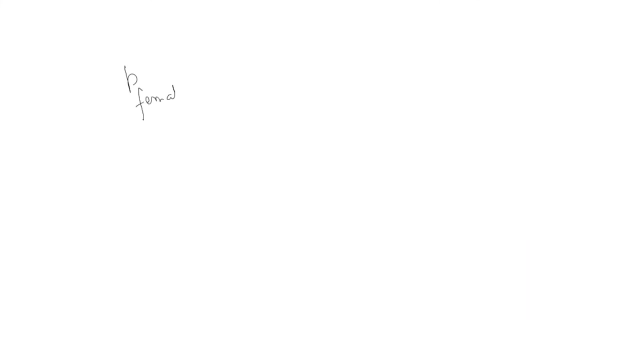 minus 0.63 square, plus 1 minus 0.6, which is 0.37 square. let me draw that out for you so that it's easier for you to understand. so probability among females watching the movie is 0.63. probability of male watch: 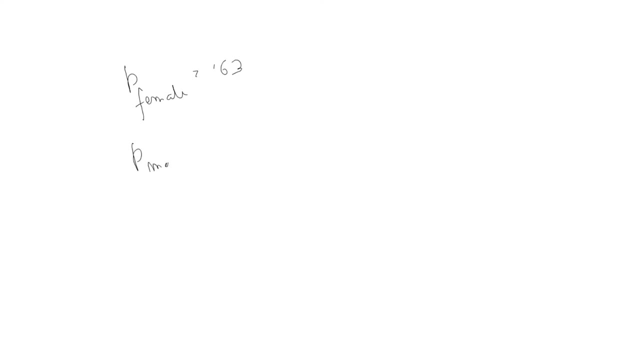 the movie is 0.37, I'm sorry, 0.43. so genie index for the female node is 1 minus 0.63 square. plus 1 minus 0.63 is 0.37 square. so this is for the female node, and for the male mnode it is 1 minus 2 minus 3.. 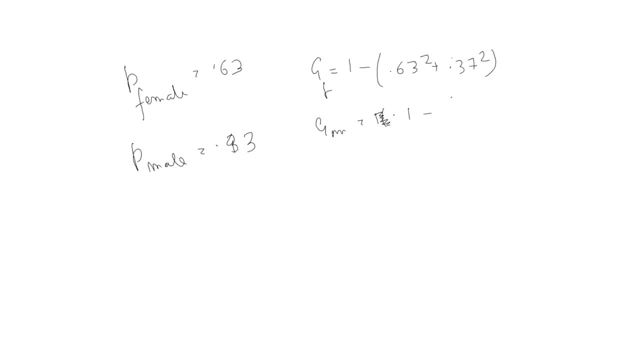 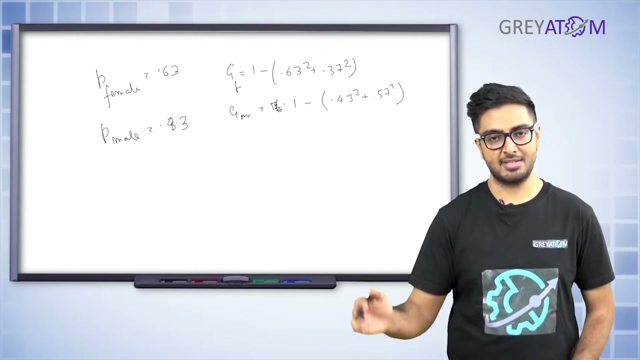 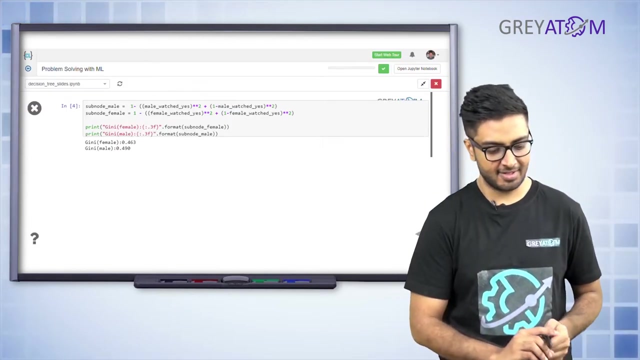 sorry, 1 minus 0.43 square plus 0.57 square, right? so this is for the male node, right? so this is basically derived from the fact that genie index value is 1 minus p square plus 1 minus p square. so now this is exactly what you have here, right? so genie index for the female. 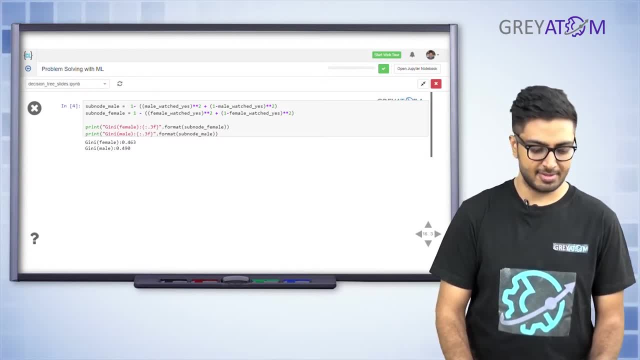 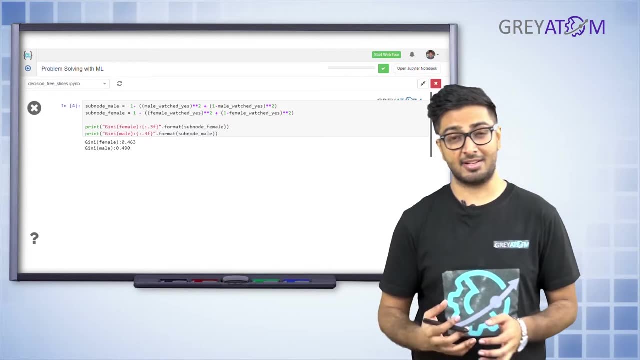 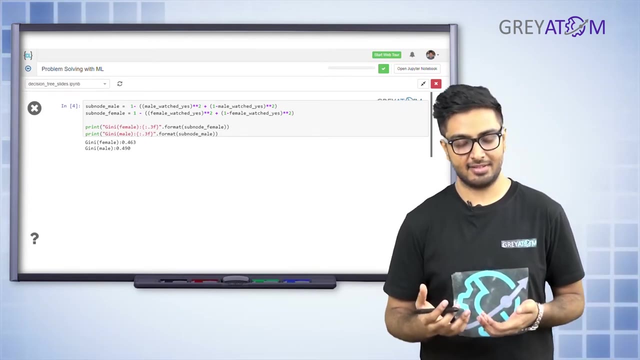 node is 0.463 and genie index for the male node is 0.490. as you can see, the male node is more impure and the female node is less impure because the female node consists of 63 percent of people who watch the movie. 63- 37 is obviously a better split than 43- 57. right, that's what we have for. 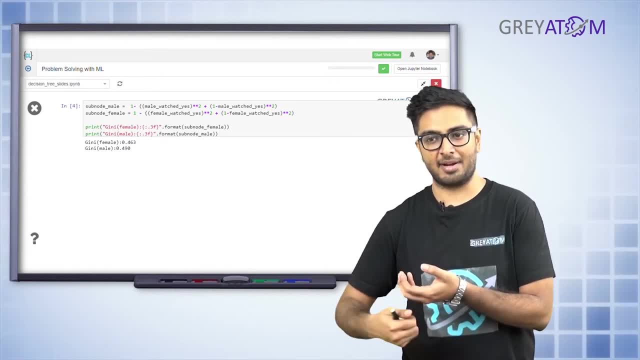 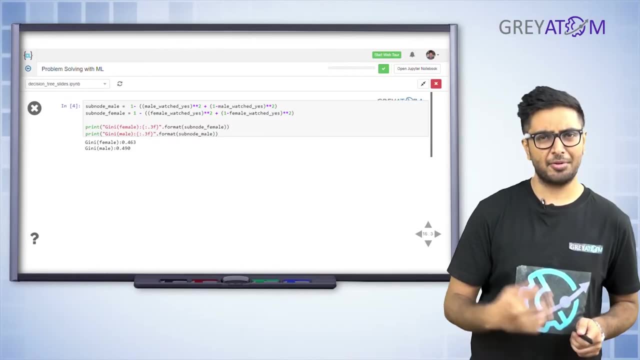 the male node. so female node is obviously better, you know, separated into ones and zeros, rather than the male node, and that's why you see the impurity score here being much lower. so now, how do you calculate the genie index for a feature split? right, because the feature gives you two. 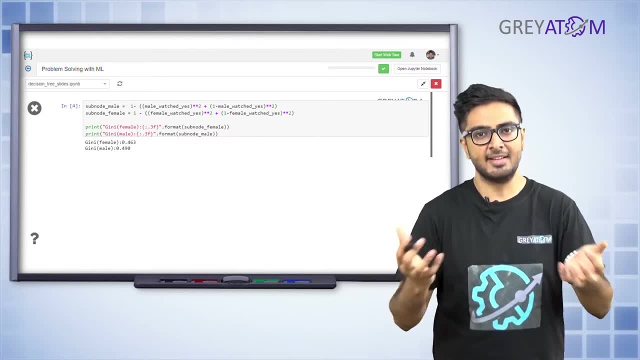 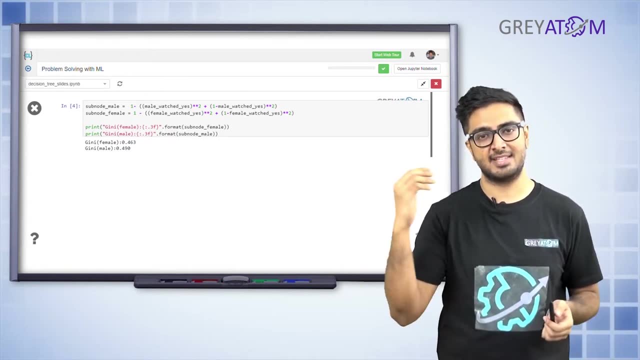 possible nodes, male and female. somehow you have to combine this right to get what is the final genie index for a gender split right. so all you're gonna do is combine them and then basically see. in the same way you combine the splits for age, employment and see which is the one that gives. 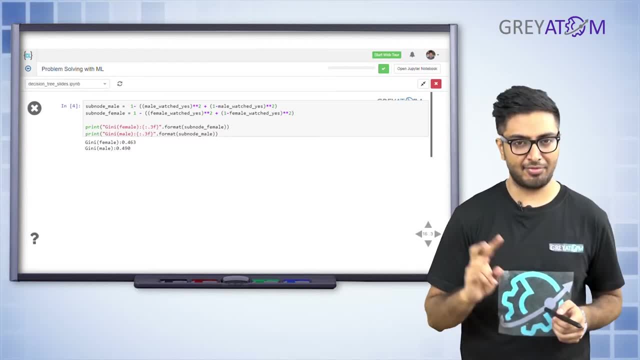 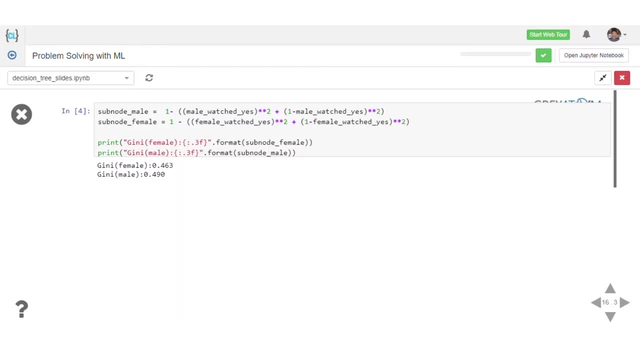 you the least impure nodes, right? so in case you have two nodes, one is 0.461 is 0.490. obviously 0.463 is less impure, 0.49 is much more impure. so but we somehow have to combine them, right. 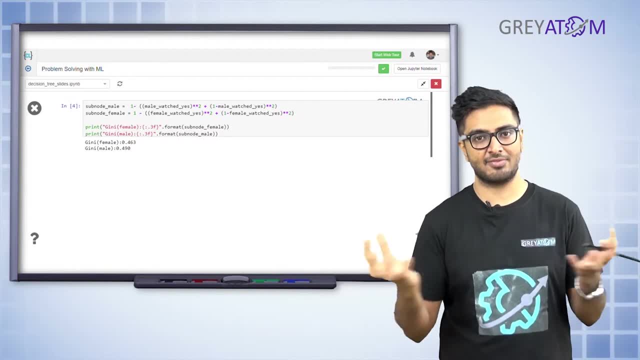 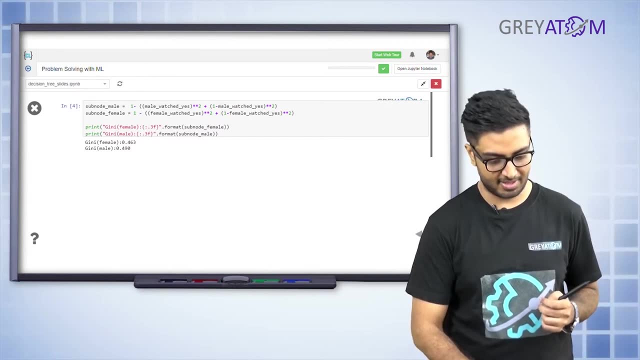 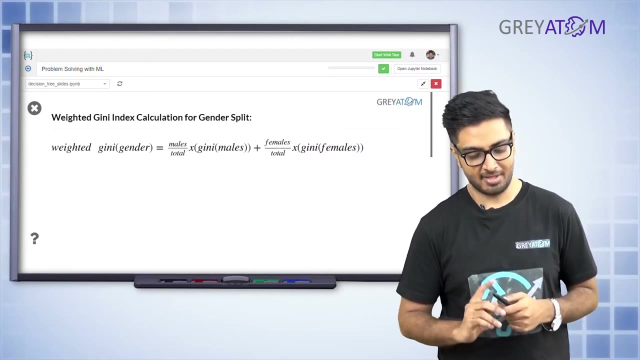 because these are two nodes and we have to somehow combine what is the final, final genie index for the gender split, right? so how do you calculate? is basically combine them using weighted average, so the weights being the total number of population in them. so in this case we have total number of males as 28, so 28 by 50 into 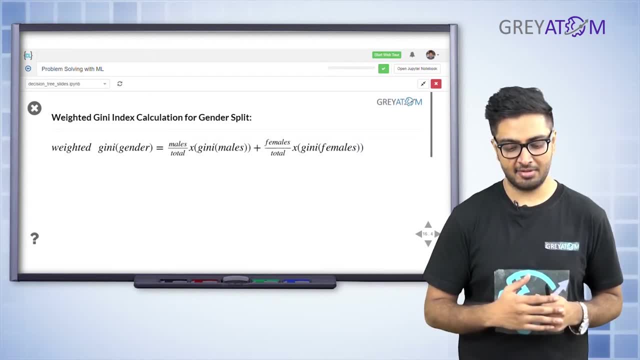 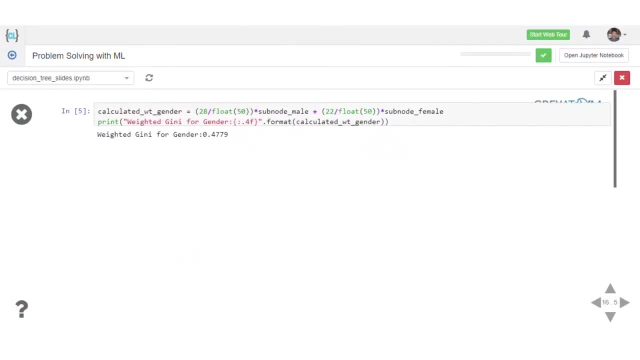 28 by 50 into the genie index of male, which is 0.490, plus 22 by 50 into genie index of females, which is 0.46. so this is what you get: 28 by 50 into the male genie index score, plus 22 by 50 into. 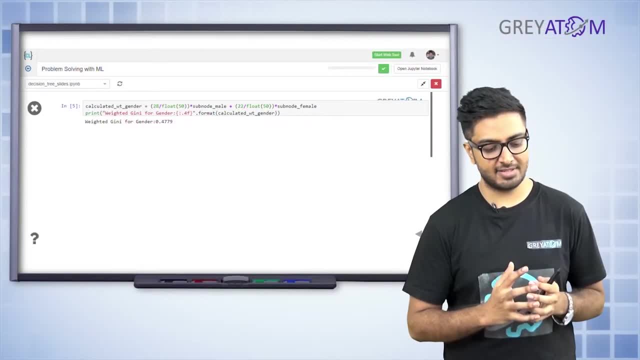 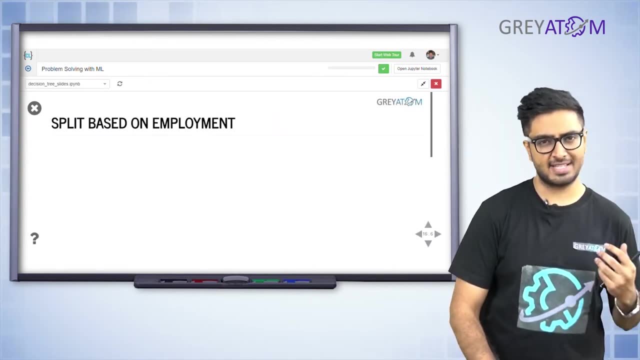 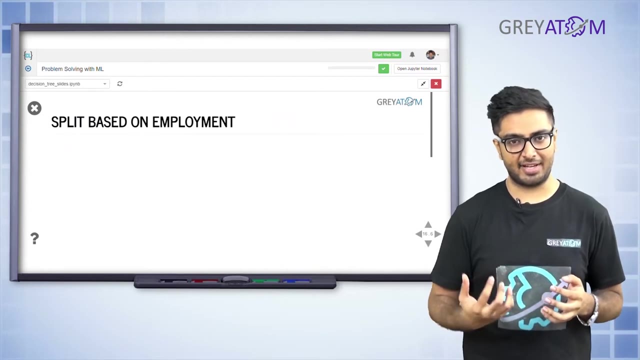 the genie index of the female node. so the final weighted genie index for gender is 0.4779. so now we'll now do this exact same calculation based on employment, and the whole idea to do this is if employment gives me a final genie number value, genie index value for the 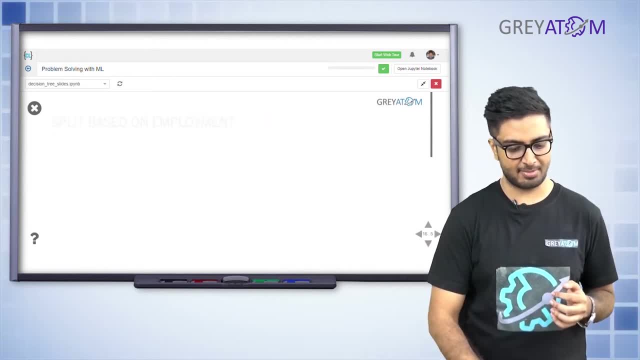 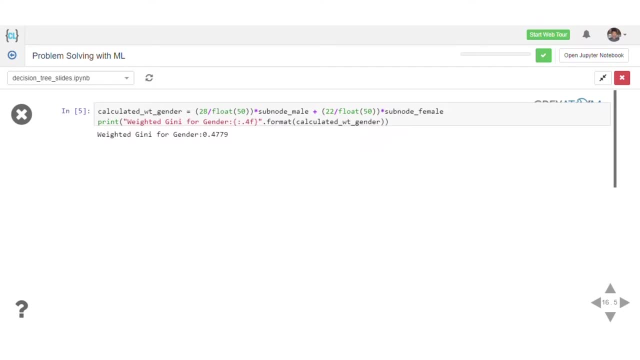 entire split as a lower number than what we have for gender, which is 0.4779. if the employment number is lower than 0.4779, we decide to go and get split with employment right as opposed to gender. but if the employment number is higher than what you have for gender, then 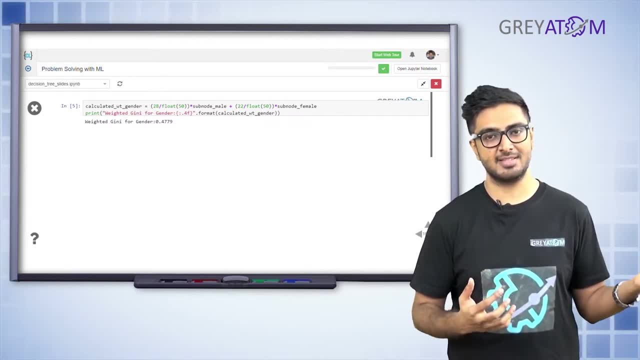 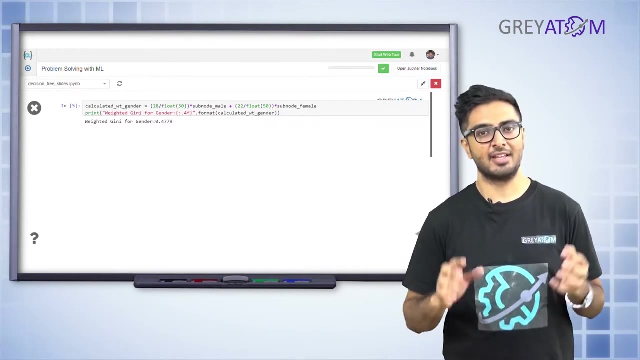 you decide to go ahead with split with gender, because then what it means is gender gives employment. employment gives you probably much more impure splits. whichever gives you the higher, higher genie index value, that is a feature split which gives you more impure nodes. you don't want to go ahead with that. you want to go ahead. 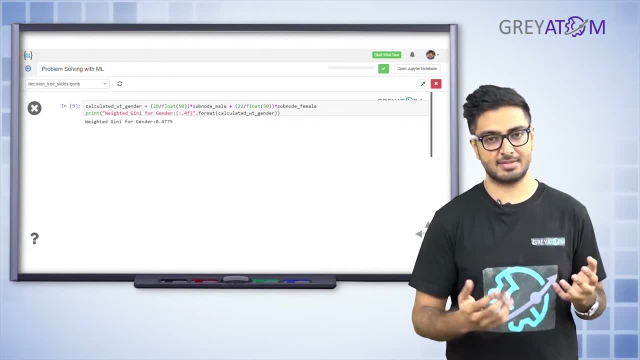 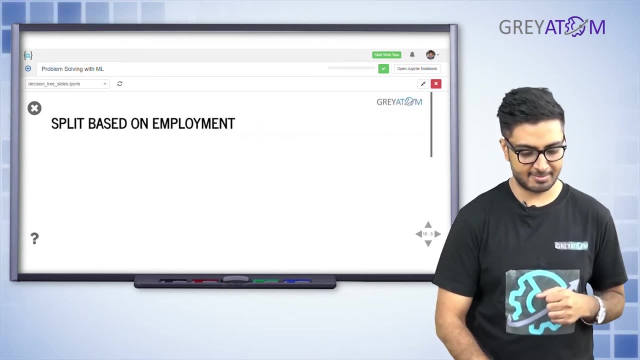 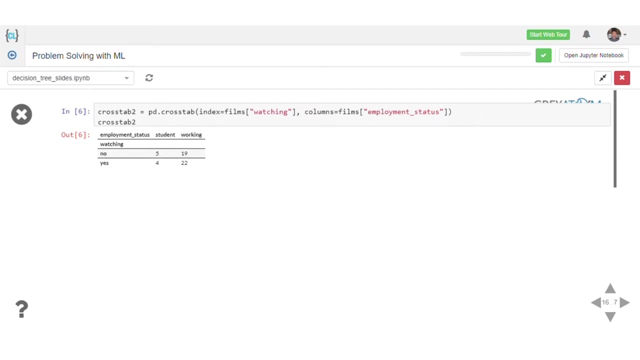 with the feature that gives you the lesser impurity score, which is lesser genie index value, right? so genie index for gender is 0.48. let's see what is the employment split. if you do split based on employment, what does that genie index come out to be? so you have the same calculation, so you have nine people. 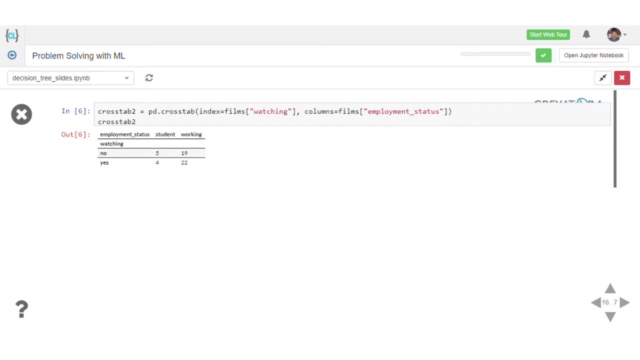 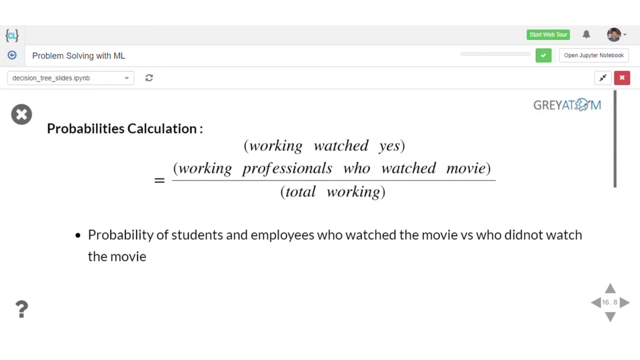 and you have 20- 41 people in one group. so out of nine people, four people have watched the movie and out of 41 people, 22 people have watched the movie. so probability of who have people who have watched the movie yes is out of. so this: 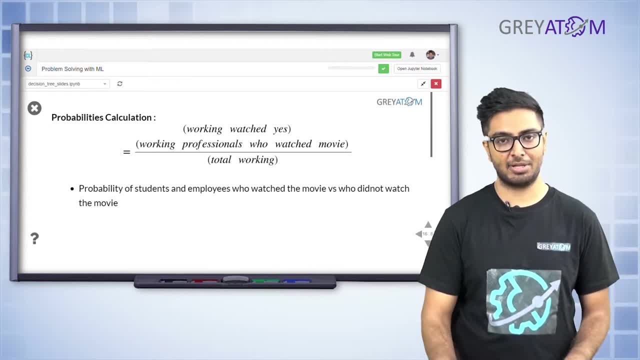 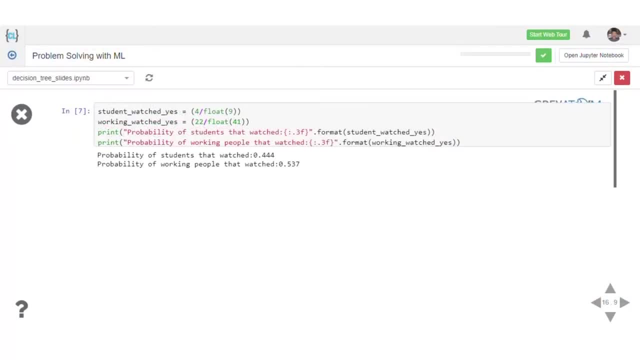 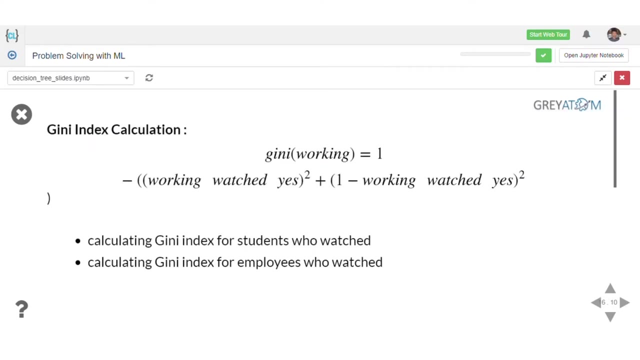 is my working profession. out of working professionals we note: out of 41 people, 22 people have watched the movie. so out of students, for people have watched the movie. so that is a roughly the probability distributions looks like this right: point four, four and point five, three, seven. so now what is the genie index for the working nodes, the 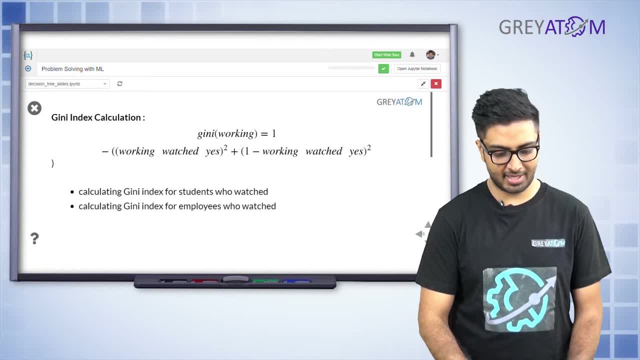 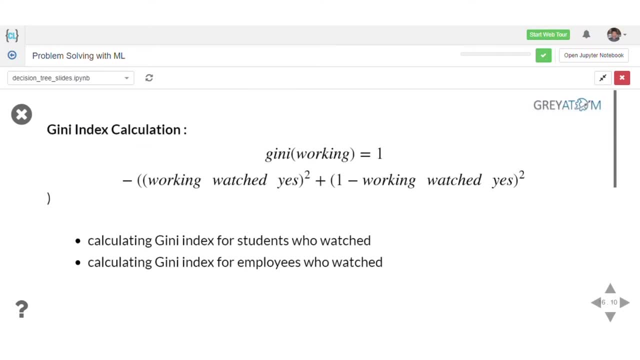 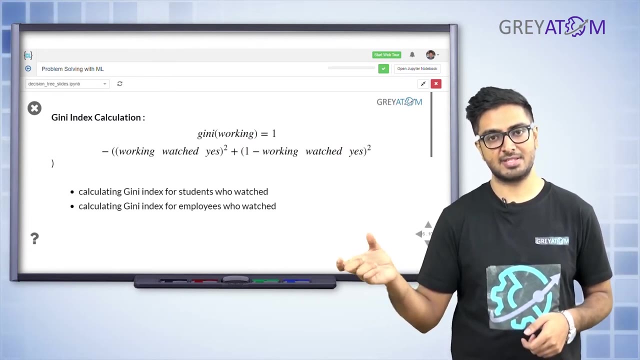 genie index for the working node is people who have watched. we're working and I've watched it, so that probability is point five three seven. point five, three, seven. so you put in plug in the value point five, three, seven here, so one minus point five three square, plus one minus point five three, which is point. 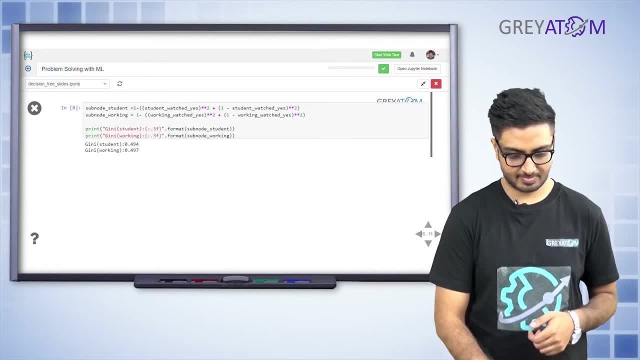 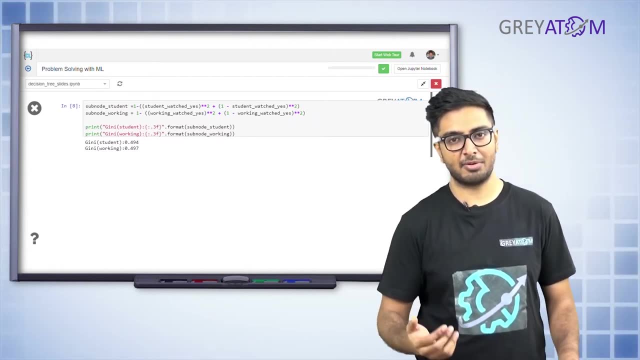 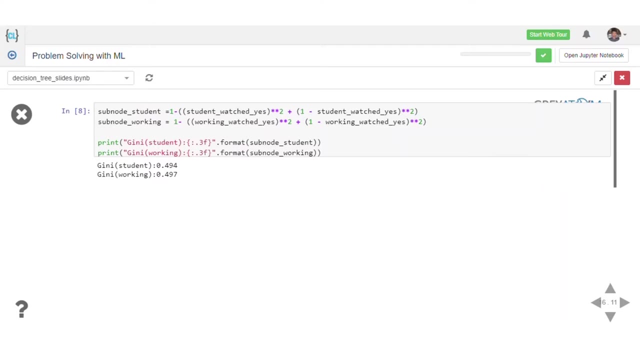 four, seven square, and you do the same thing for students as well. so student the population, the display, the probability of someone watching the movie was 0.47, I guess. so one minus point four, seven square, plus whatever that comes out to be. so genie index for students and genie. 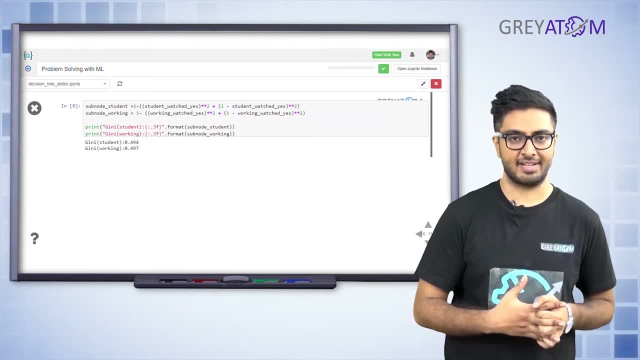 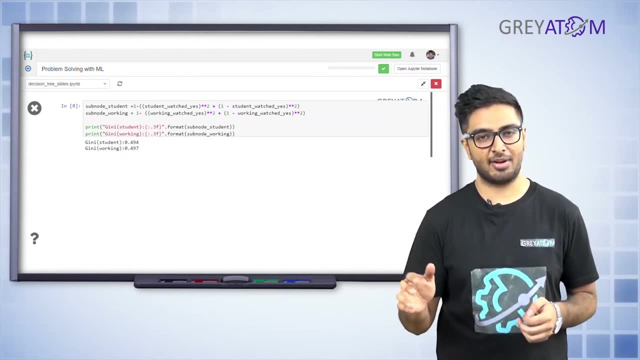 index were working at point four nine four and point four nine seven. now you can clearly see that both the nodes are almost impure right. the most impure node can have a genie index of point five value and here both the nodes are almost as good as impure right, because the student has a 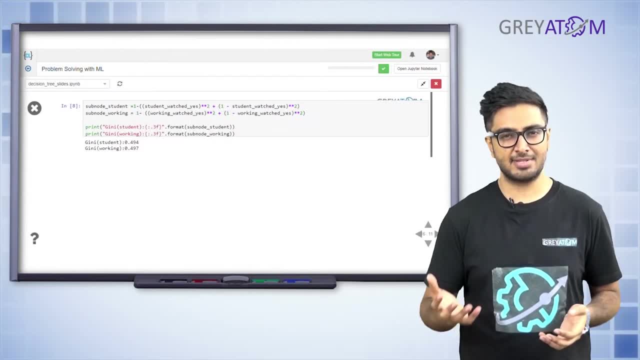 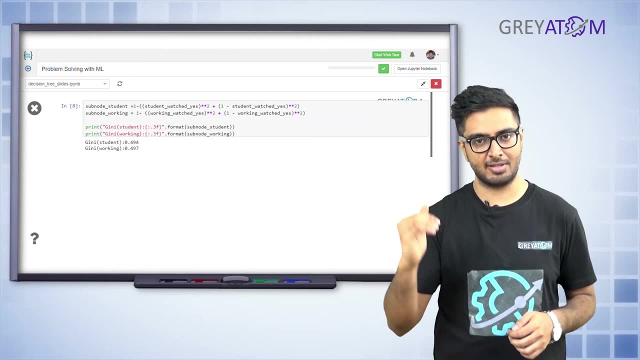 0.494 and 0.497, so which is basically to say all of both the nodes are 50- 50 splits, and this is something we have already seen earlier. right when we did the tabulation of all the possible splits, we saw that employment was not a good option because it had a very close to 50- 50 splits in. 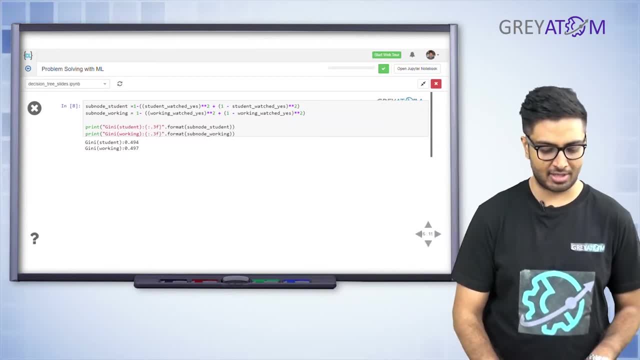 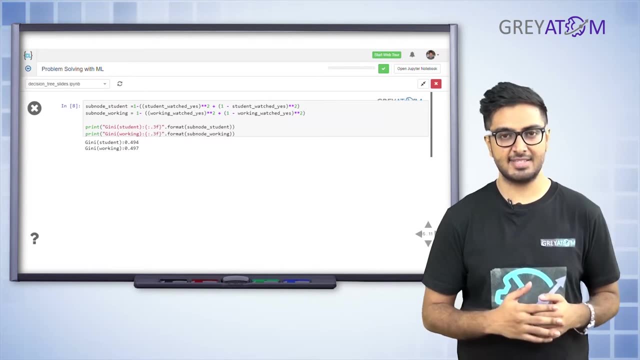 both the cases, both the nodes, and that's exactly what you see as quantified here. that was an intuition that we had: that employment is not a good idea because it gives you a 50: 50 split. in this case, we can see that employment is a is obviously as not good at is because it has given 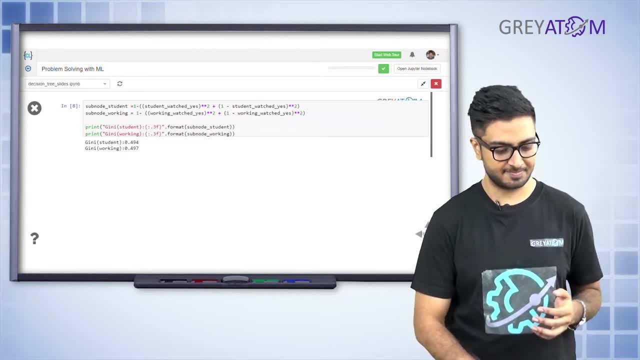 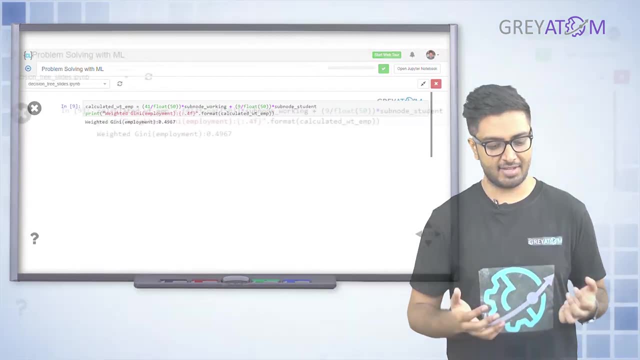 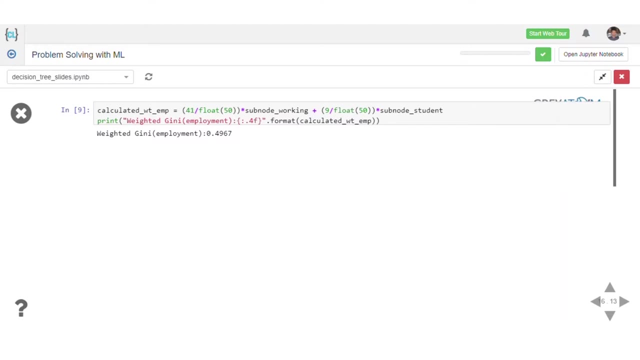 you a 0.5 genie index for both the values, both the splits, sorry, for both the nodes. so now weighted genie index for the employment is basically given as the same way: 41 by 50 into the genie index for students- sorry- into the genie index of working people and 9 by 50 into the genie index for 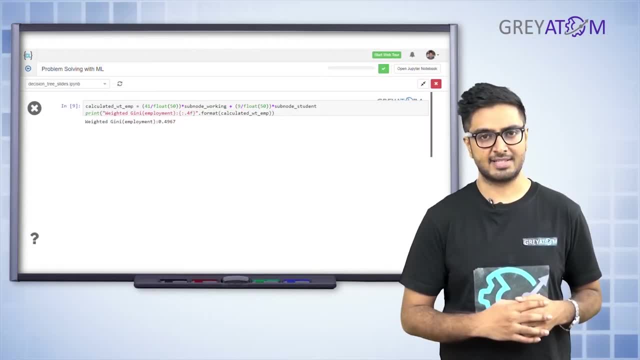 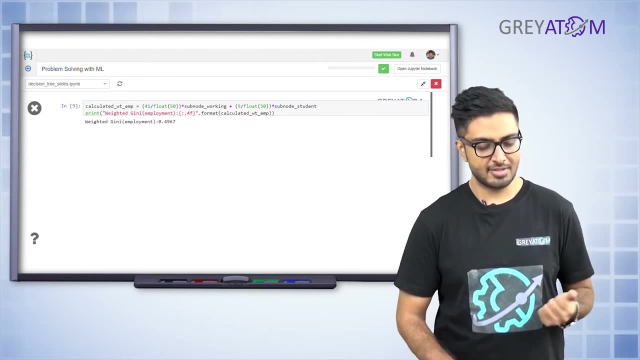 students and that comes out to be somewhere on 0.4967, so which is obviously much higher than the genie index which we had for gender. that was a 0.48. so obviously that means that employment gives you more impure node because the genie index is higher as compared. 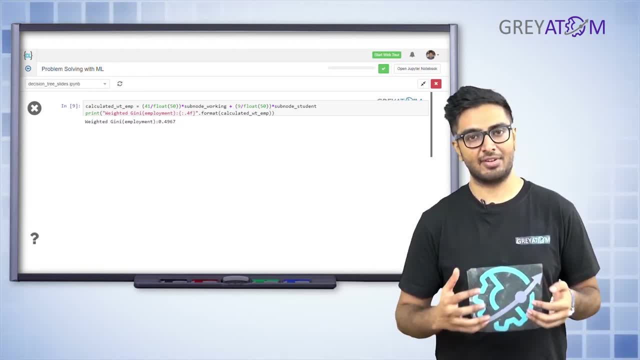 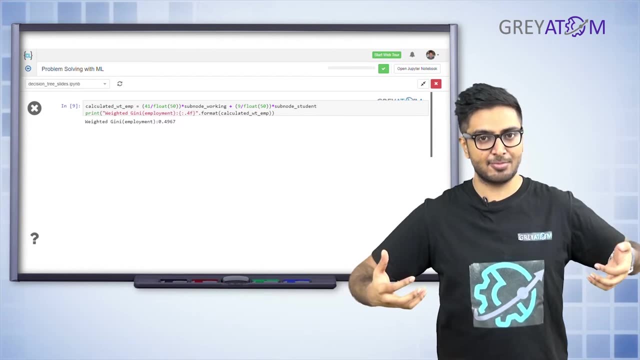 to gender, which gives you less impure nodes. so by definition, by the design of the algorithm, we are going to go ahead with gender, because that gives us more pure split. it separates out your ones and zeros into two distinct classes, and that's exactly what we want here. so that's. 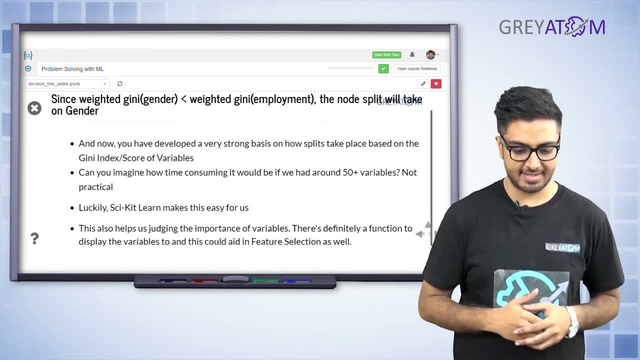 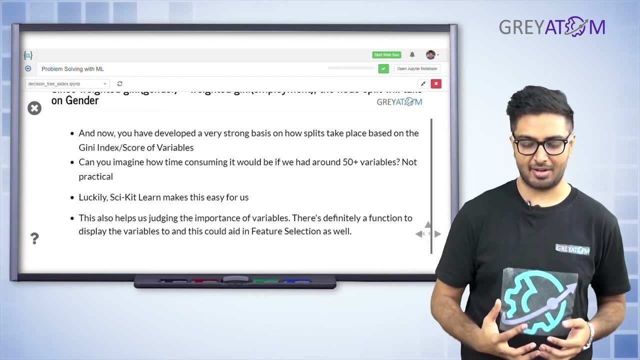 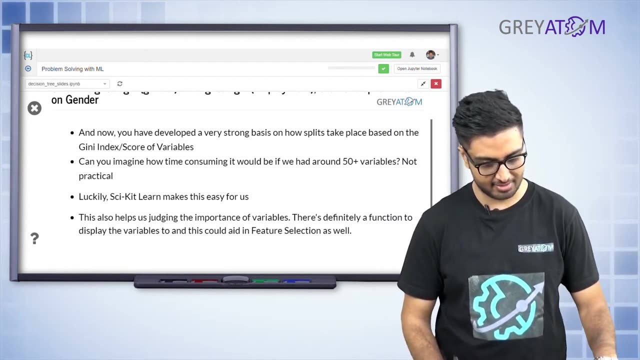 what you see here on the slide. genie on gender is less than weighted genie of employment. the node split will take place based on gender. and now you have developed a strong basis on how splits takes place based on the genie index and score so at each step. so now to kind of formalize the algorithm for you. 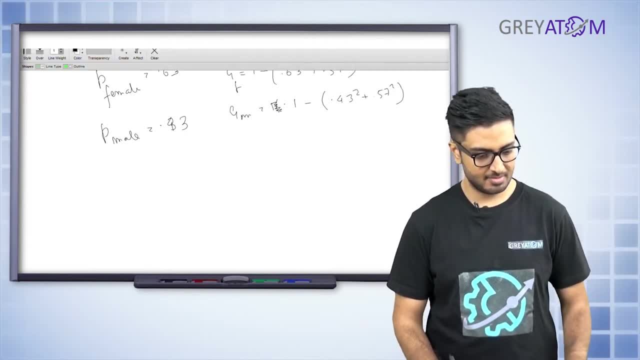 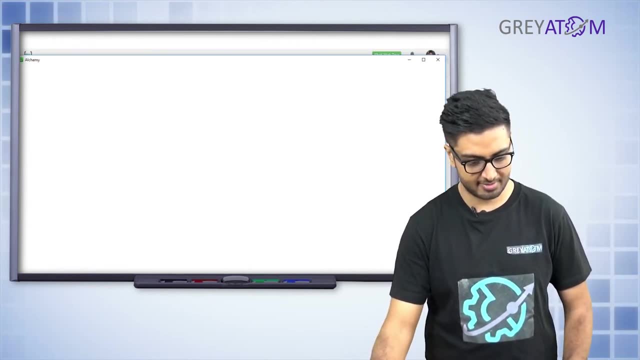 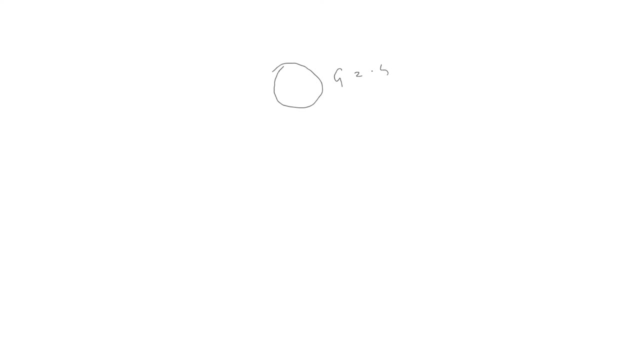 let's go back and draw this for you. so let's consider this dunkirk example. only so we had started off here, sorry, yeah, so this is your initial node. this had a genie index of 0.5 almost because it was a 50: 50 kind of a split. 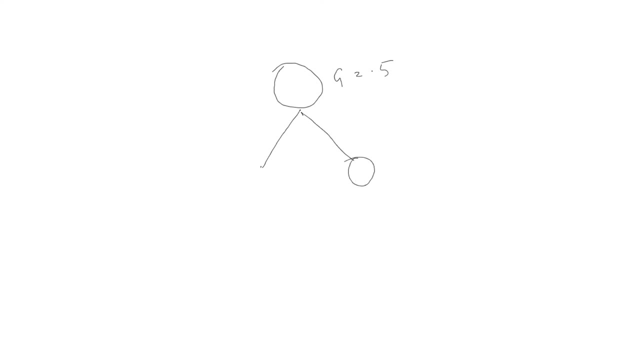 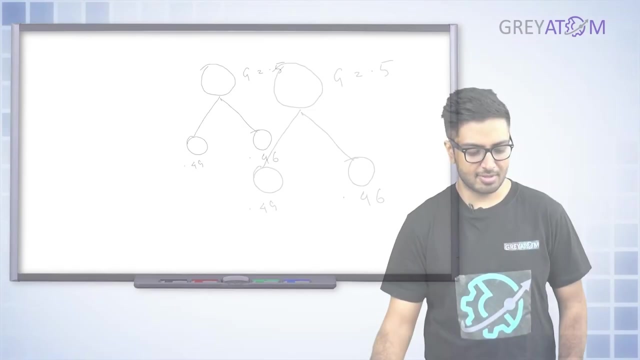 so from here, based on age, you can see that you have reduced down the genie index. so one has got a genie index of 0.49, the other has got a point genie index of 0.46, right, so now this genie index are obviously not close to zero we want, because zero is exactly where we want to. 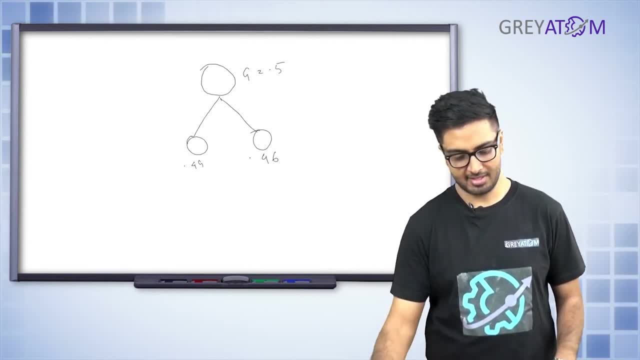 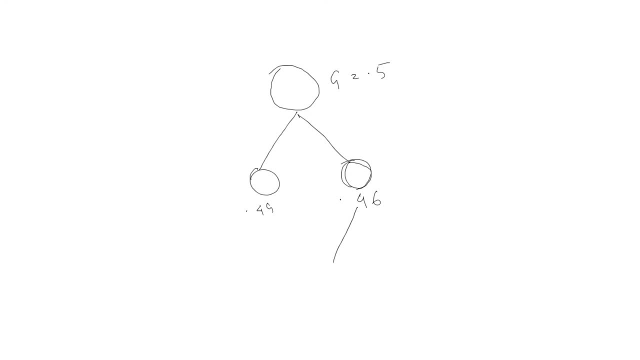 stop, because zero means that we have reached completely pure nodes. but these are not pure. so we again look at all the three, all the three possible option to split here as well. right, so this is a genie index for gender. so let's say this is a male node and this is this is the female. so this was a male node. 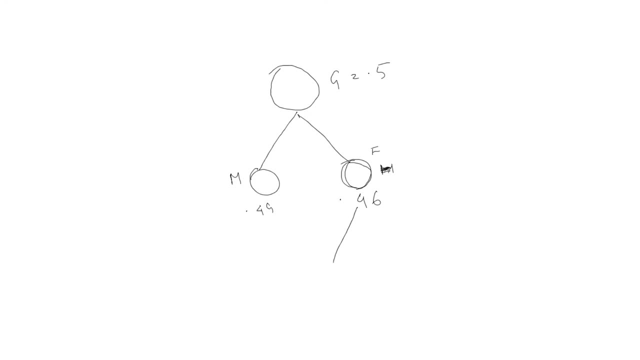 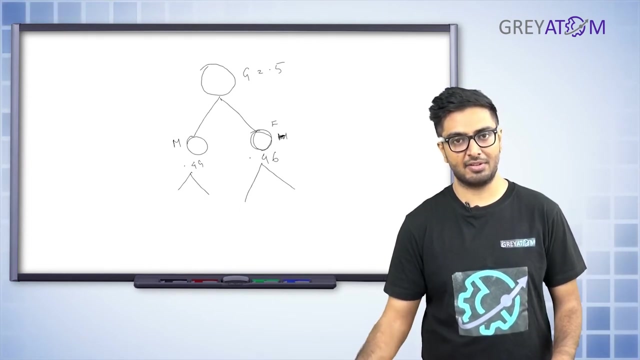 sorry, and this is the female node right. so, on the female node, we want to split them again further, and so we want to do for the male node as well. and again, while we're splitting the female node further, we again gonna look at all the three possible features, which is gender, age and 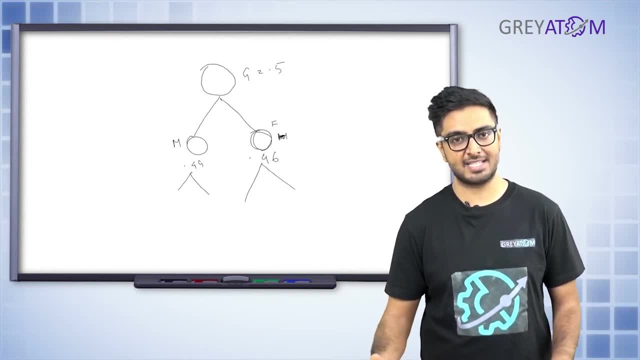 employment and decide based on that which is the next best option to again split at this stage. right? so just because age has been split here doesn't mean we don't consider age here. if age has been considered here, we again gonna consider all of the three possible features to split on at. 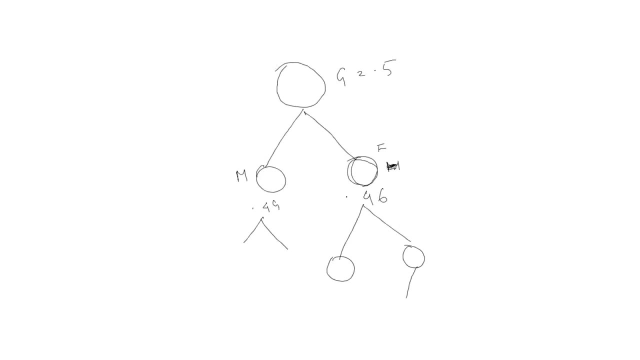 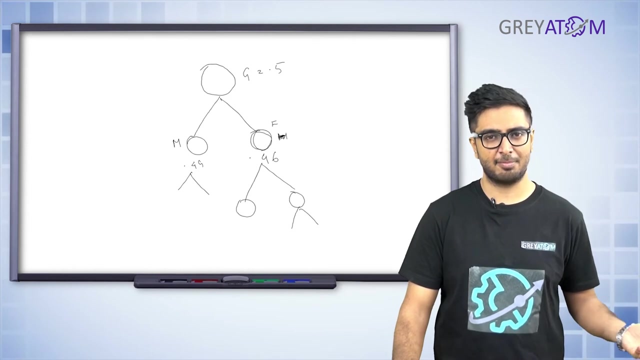 this stage as well, and then we are gonna keep on doing this right until our genie index value basically comes down to one. sorry, it comes down to zero, because zero is basically the point where we say that we have reached a completely pure node. it could be of people who 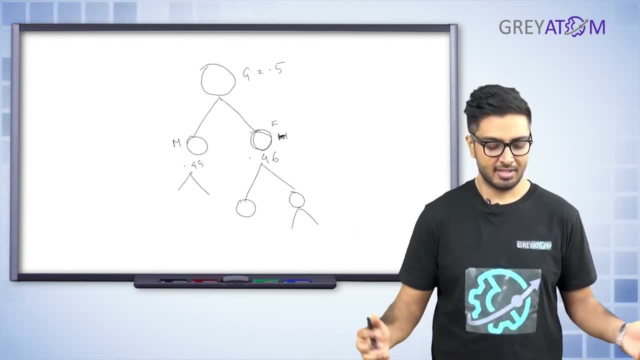 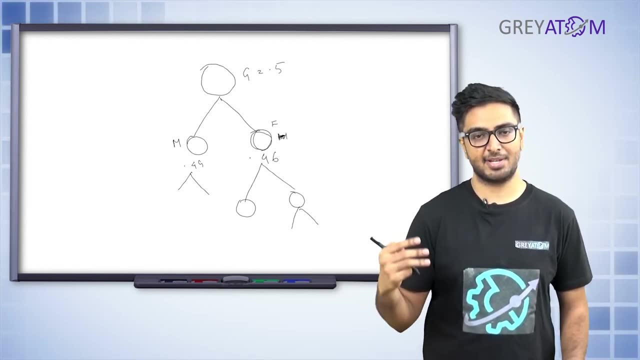 have either watched the movie or it is basically people who have not watched the movie. but if we keep on doing this iteratively, at each step you are going to consider all the three possible splits, and for all the three possible splits, you are going to consider the genie index, and then you're. 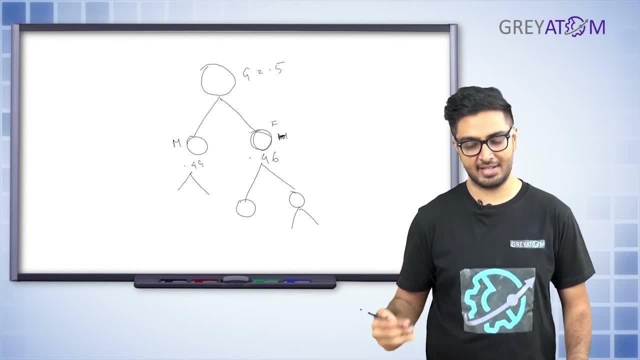 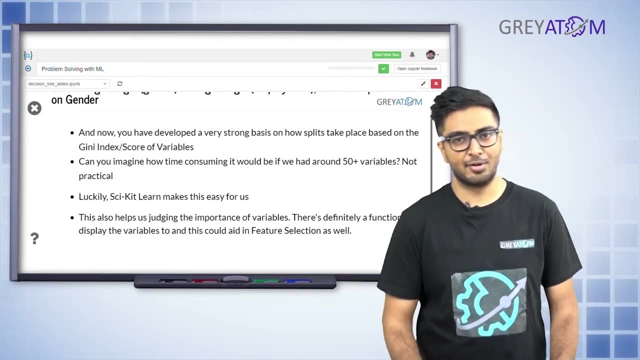 going to see which is the split which gives you the least possible genie index and based on that, you kind of take the call of which is the feature you want to go ahead and split with. so obviously good for you is that, for most of the algorithms that we have discussed and we have talked about, 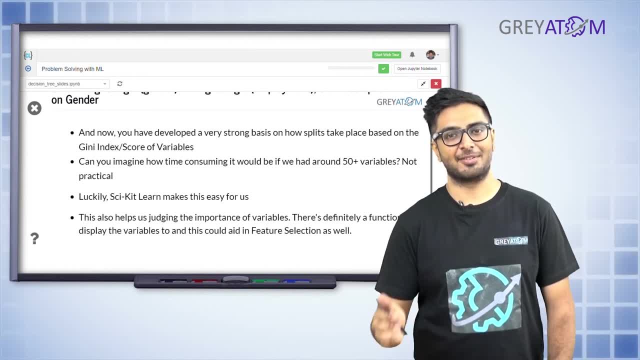 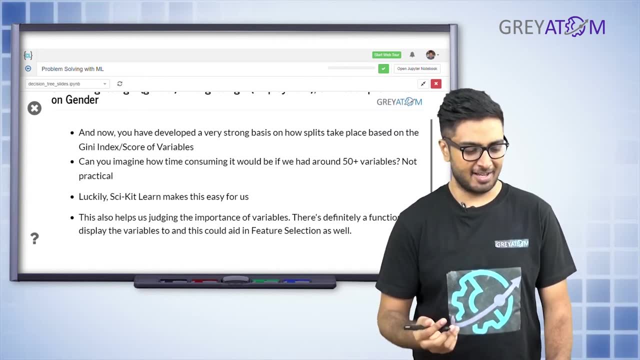 uh, it offers you api for doing all of this. it's not like you have to calculate all of this at every step of every node of the calculation. you can easily skip all of this. uh, but obviously, as i have always been talking about in the lectures and here, as 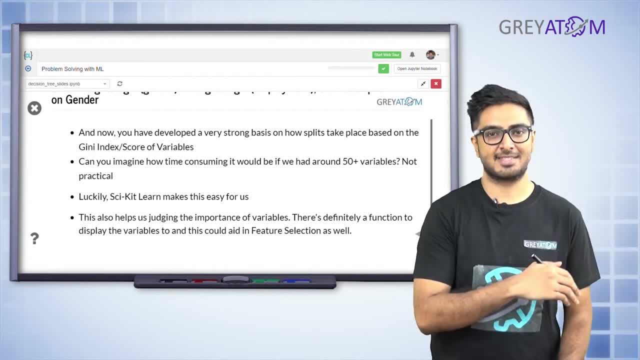 well, it's easy to kind of, you know, just go back to scikit and just put this as an api and just go ahead with it without learning and without understanding all of this. but understanding this is extremely critical because sometimes, when your algorithms don't work, you kind of want to go. 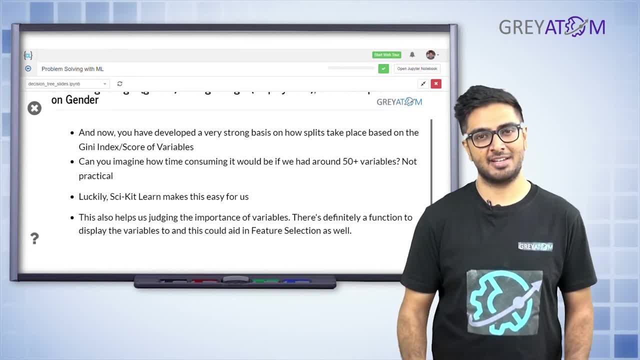 back and debug them right, and if you don't know exactly how a genie index works, it would be extremely impossible for you to kind of debug why your algorithm is not performing as you expect it to be. so don't, don't, don't, don't, don't rely on the fact that scikit offers you an api for doing. 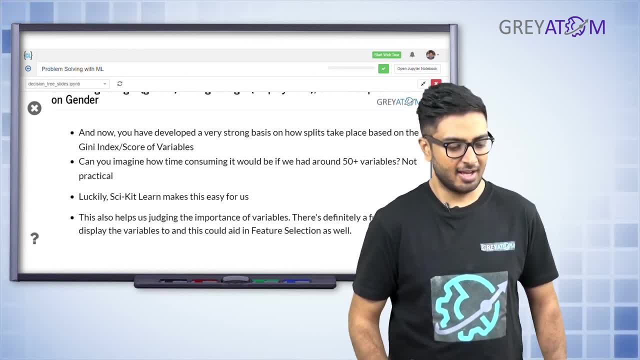 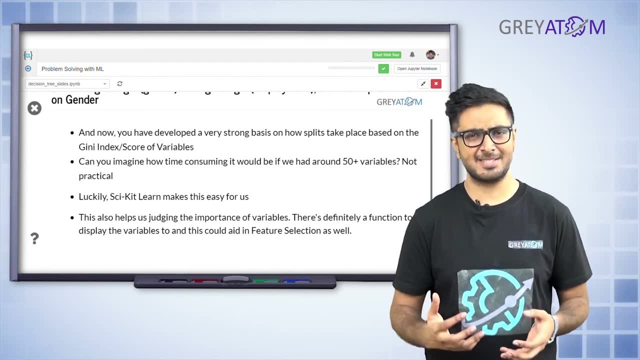 all of this without you calculate, needing to calculate all of this. uh, that is good, that is convenient, but that doesn't mean you can skip the part about understanding genie index and, frankly, this is all simple sense. this is not as complicated as a linear regression or anything. 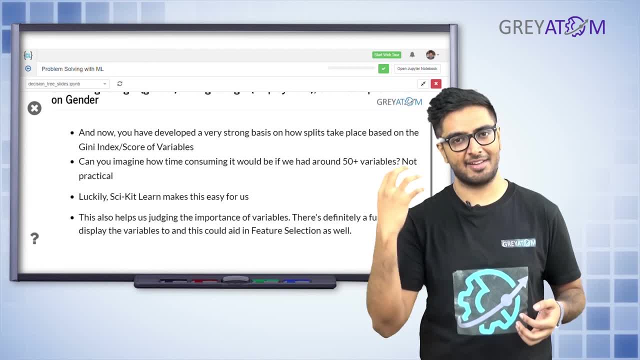 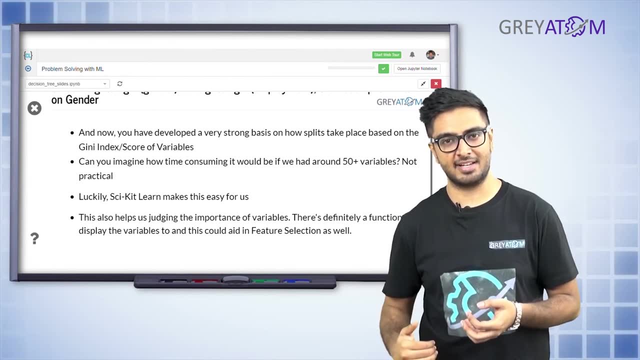 you have got an algorithm which measures, measures an impurity split, and at every step you're going to measure the possible feature, all possible features you're going to consider. you're going to consider which is the feature that gives you the least genie index of the child nodes. 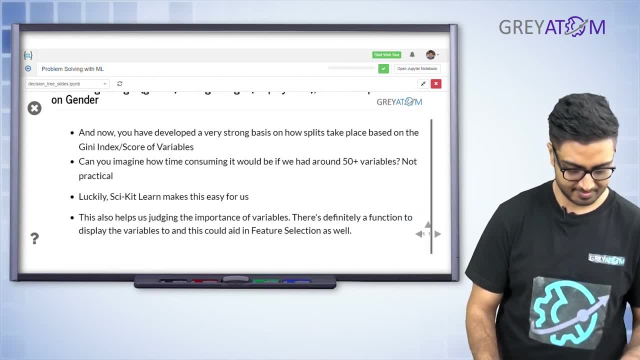 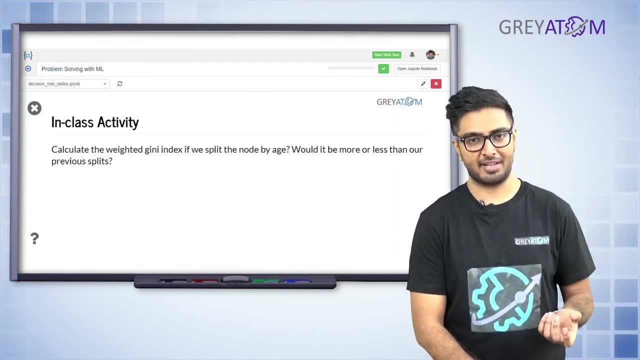 and you're going to go ahead with that feature. right, that's very intuitive. so now we are going to cover chi square index. so obviously you can want to probably take a minute and understand about how you would calculate the genie index if the split had been done by age. right for age, there were two possible. 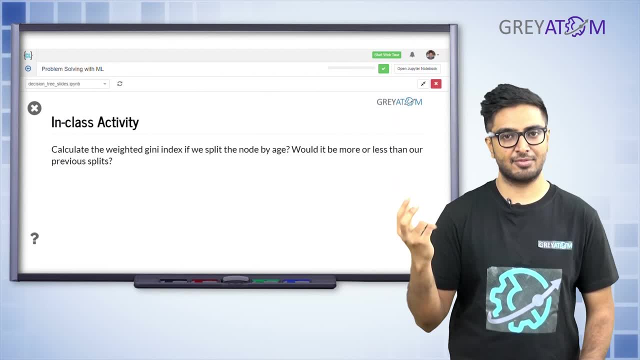 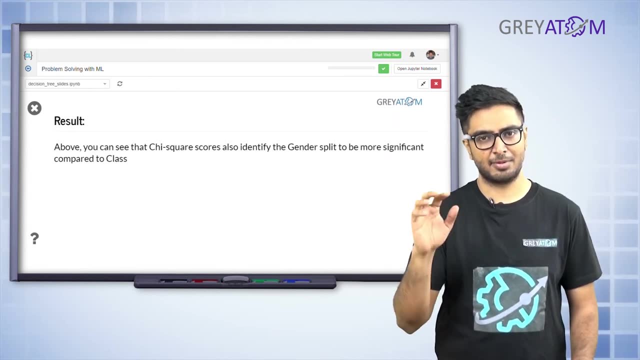 splits possible, 28 plus or 28 minus. so for each of those values you want to calculate what is the probability of someone watching the movie. and then, plugging in the probability of someone watching the movie, if someone is 28 plus, what is the probability of someone watching the? 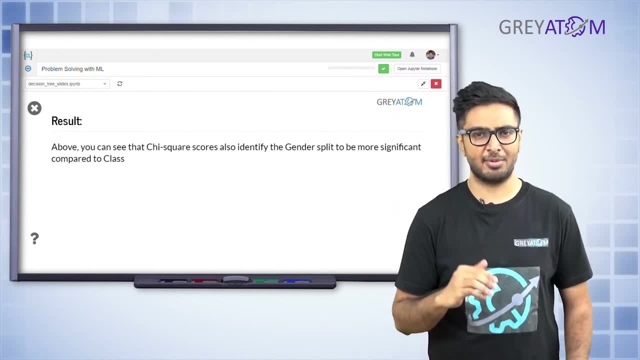 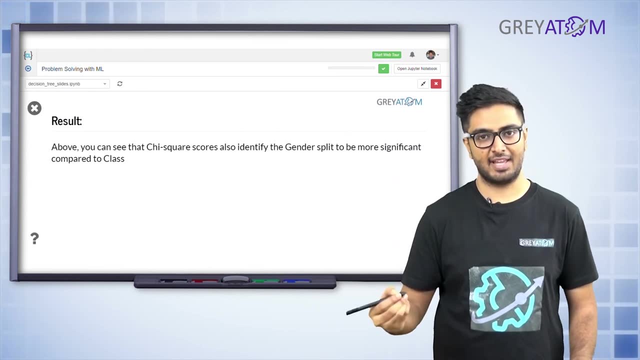 movie if someone is not 28 plus, and then plug that formula into the genie index and see what is the genie index that you come up for the age y split right and then see if ages of time do you want to split up based on age versus.